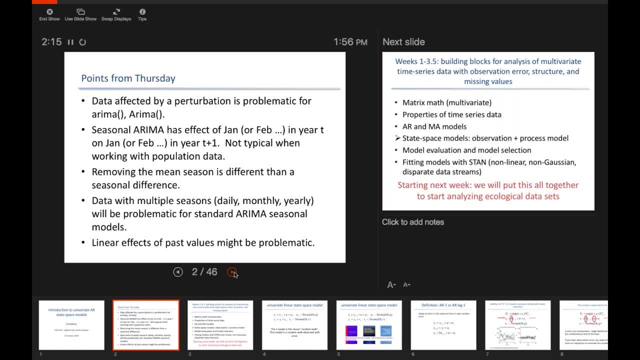 You can have that covariate effect, multiple future years or multiple months in the future year. Okay, And then another big point somebody asked: is removing the mean season the same as a seasonal difference? And no, It's definitely different. And think about that example where the season is like increasing, like this: 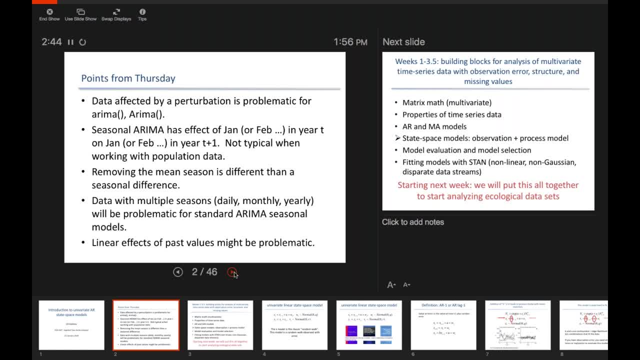 And if I subtracted off the mean season there, then I would still get a seasonal cycle that was big on this end and then it's smaller on this end, because those seasonal cycles are big here and they're small here, And I didn't mention this, but it's something important to know. 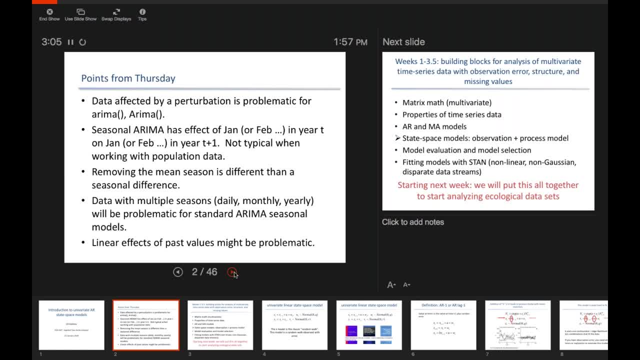 Is that? Is that, if you have data with multiple seasons, so that would be like you had, let's say, daily data and you had a monthly cycle, had something to do with, say, the tide cycle, and then, on top of that, you had a yearly cycle. 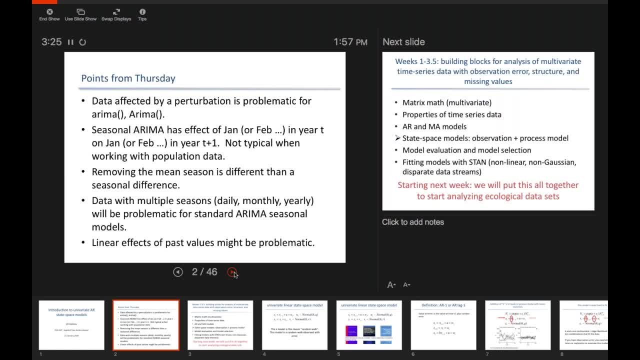 So this would be really common for us, right? if we had monthly or if we had daily data and it was working and it's in an ocean environment. It would be really common that we have a monthly cycle. Okay, So we have a monthly cycle having to do with tides and a yearly cycle on top of that. 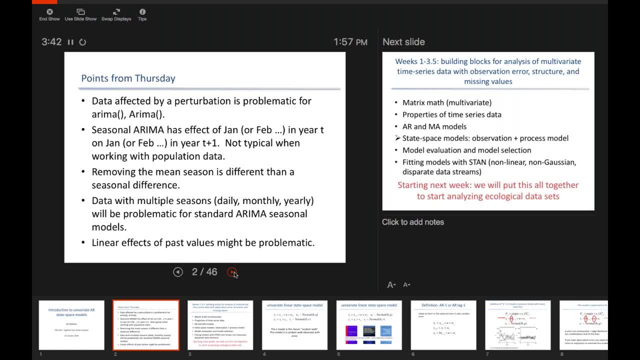 If you have that kind of data, it's going to be problematic for the standard seasonal models. There are arena models that you can apply that have multiple seasonalities, but it's not the standard stuff. Okay, Great, Move on Okay. 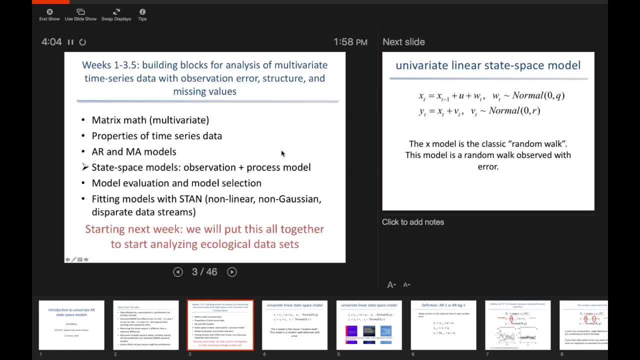 Great. So let's go into something new today We're going to talk, now start talking about state-based models. So now models that have observation error. So far what we've been working with these arena models: they don't have observation. 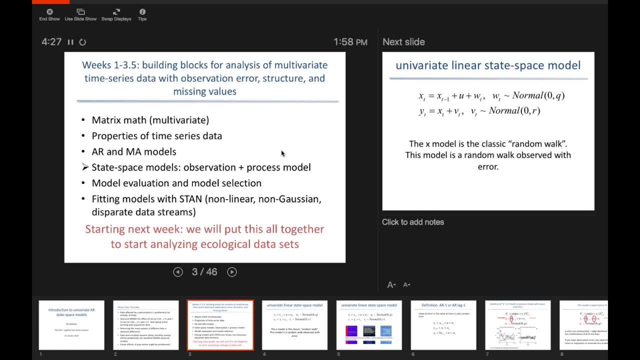 error. It's like we're modeling a process where we're modeling the value of an event and we're modeling a model: Okay, our observation as a function of the observations in the past. now, with states-based models, we're going to back up and say: well, our data are. 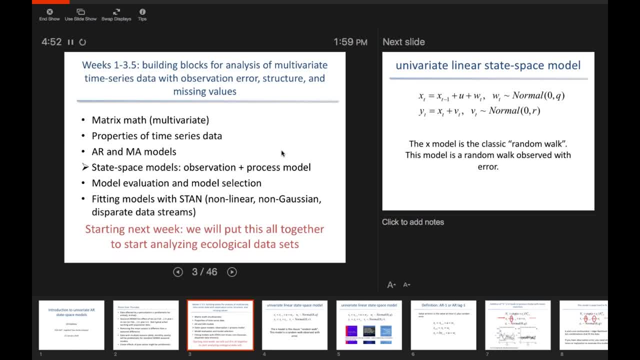 observations of an underlying process and our observations have error. so we can't, or we don't want to directly say that our observation is a function of the observation in the past. we don't want to do that directly because there's all this error in there, right? so the observation in the past might have been. 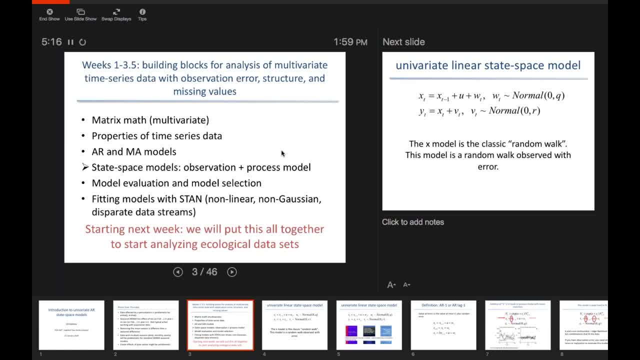 really low, not because the population size is really low, but because the river was really cloudy and we couldn't get very good measurements right. so it was low just because of observation. so we'll be talking about the observation in the past, and then we'll be talking about this class today and on Thursday, and then we'll move into model. 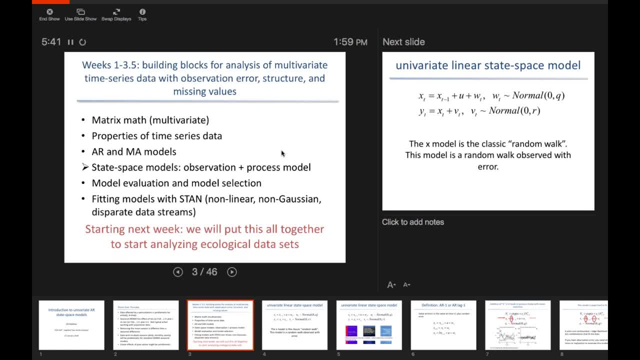 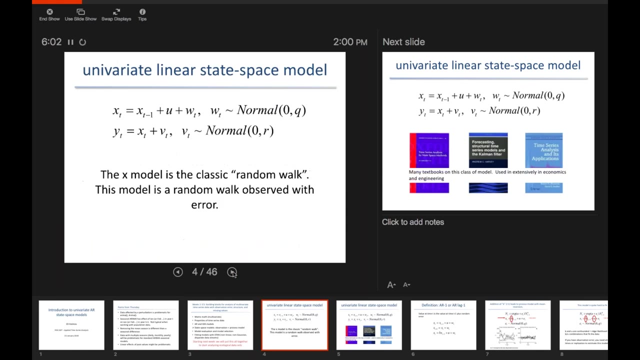 evaluation and selection, and then we'll start talking about how you can fit these, this class of model, with non-linearity and non-Gaussian errors, and once we do that, we'll start really digging into. okay, let's do some ecological analyses here as well, okay, so this is about the most simple state space model that you can come up. 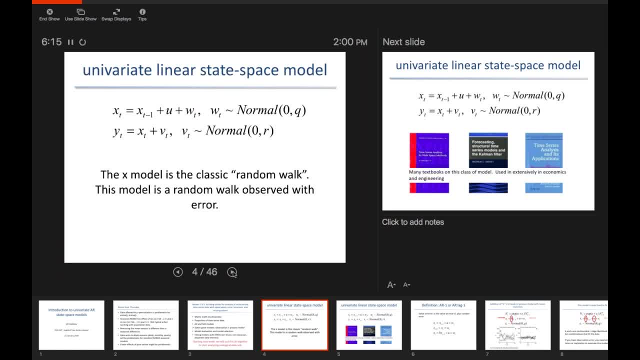 with. that includes a random walk. we have the X part is the process. so there's something that we're observing and you know it's a random walk, So that's a random walk. right there You see that time dependency: there X at time t is a function of x at t minus one. 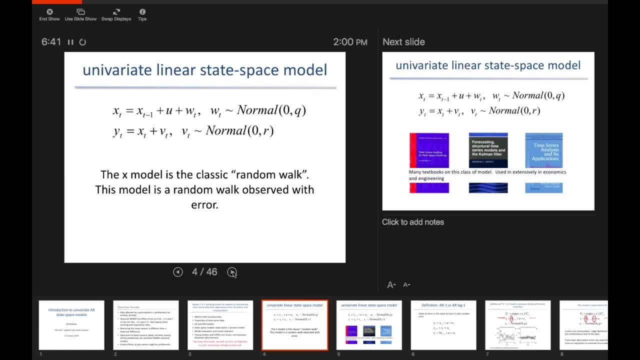 There's no b term in front of there. So since you just see that term appearing without any parameter in front of it, you should recognize that that's a random walk. It's just going to kind of wander off And it's got this u term here. 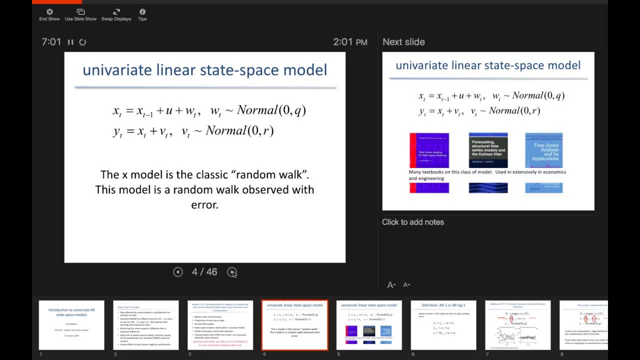 And what that means is it's going to tend to go up If that's positive. it's going to tend to go down If it's negative. that's our process. Our process is a random walk, but we don't see that. 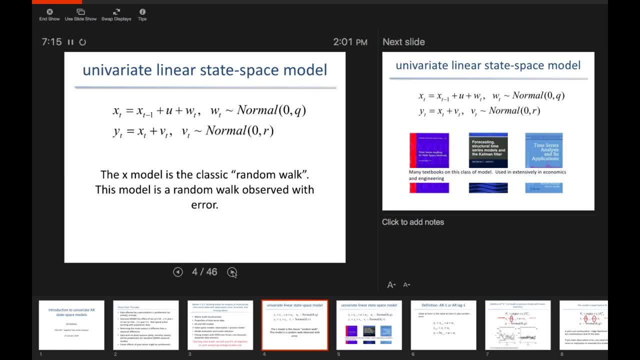 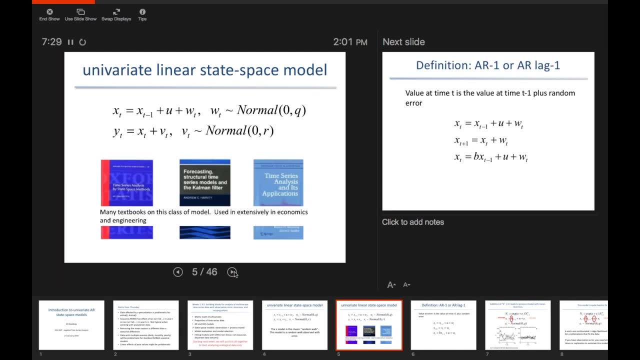 It's hidden. What we see are the y's, And the y's are the hidden process plus some error. So we observe the hidden process, but it's obscured by error, So it's a random walk. This class is extensively studied in economics, engineering. 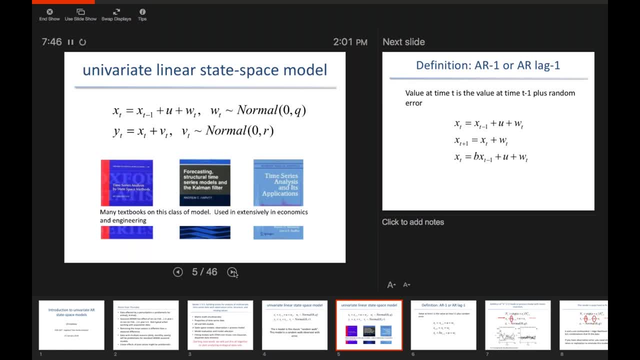 and these are three textbooks that all of us have on our desk. These are some of the classic ones, but you'll find this in lots and lots of you. You'll find this in lots of you. You can find this in all your courses. you'll find this in all your courses. 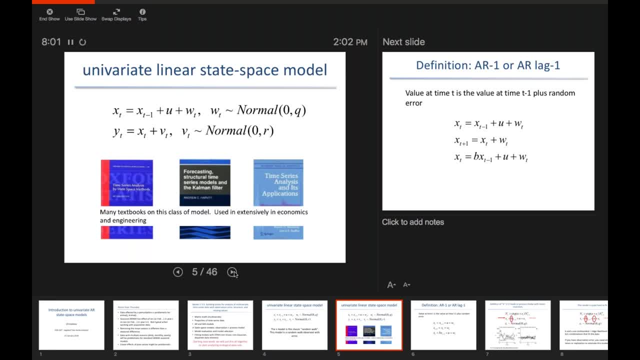 you'll find this in all of your courses, But if you just Google state space and textbook, you'll find many examples. yes, I just I think. probably all of these are listed on the class website and Google references. This is the main one I use. 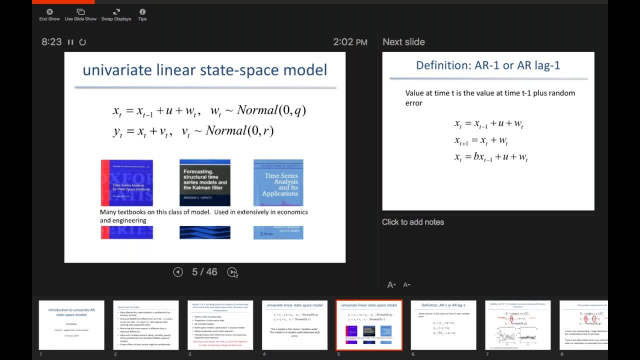 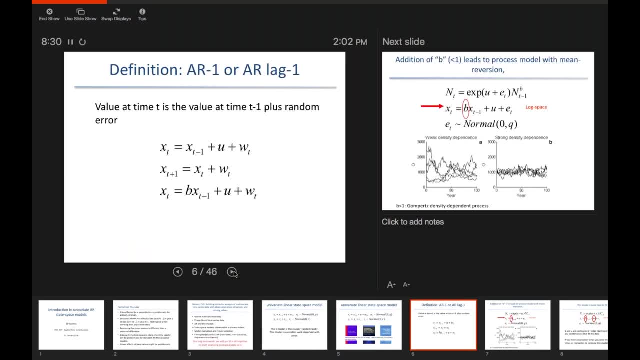 I think you may use that one more. No, No, I think that one's probably cool. These are so, I told you. the Xs are your process, And here are three of the simple process models that we've been looking at so far. 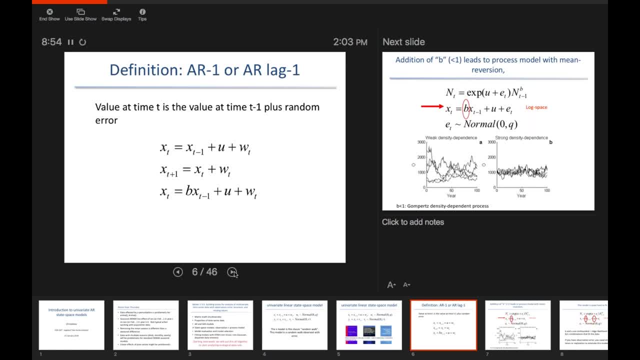 And we'll be playing a bit with these today. So that's the random walk I was just showing And it's got the trend. You could also write it this way. The only thing that's changed is it's T plus one and T. 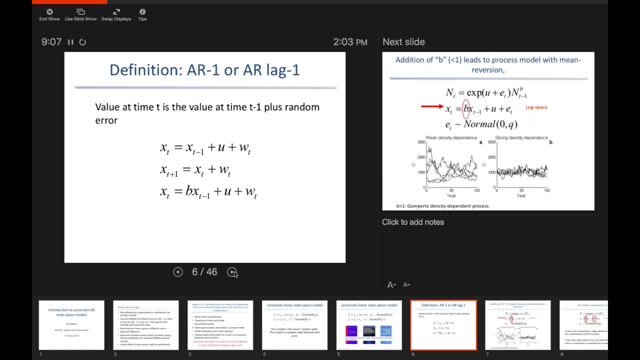 I note that because in many textbooks they write it that way, because T plus one is exactly the same model. This is missing the U, so there's no trend here. And then the other one is this one where we have this V here, in that V is between minus one and one. 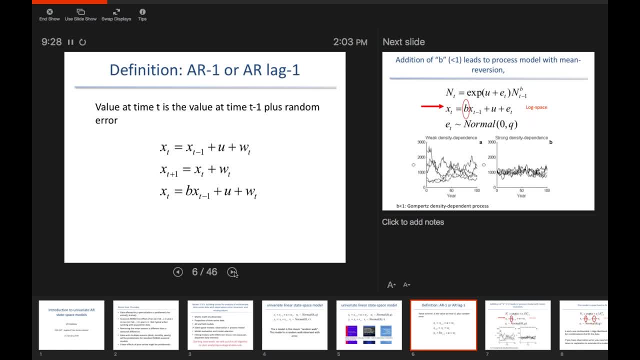 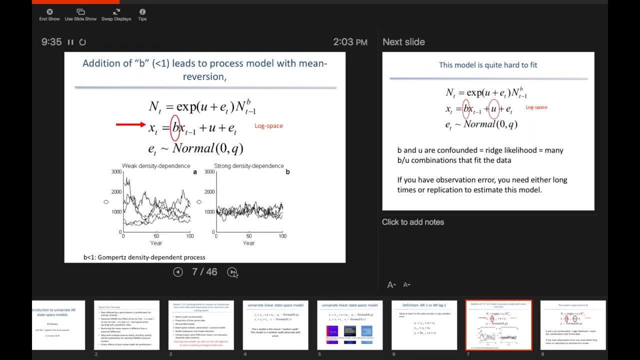 Then we have a mean report burning process. it's going to be something that's going up and down around the lobe. Okay, in ecology this model is also called the Gompertz model and it's one of the models of a density dependent process. and if you look in ecology, 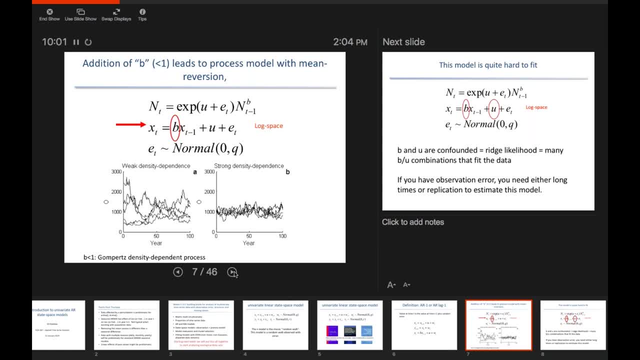 textbooks on density dependence you probably see the model written as the top. So n is population size and population size at time. t is some function of the population size at t minus 1 and that beta term is indicative of the strength of density. So density dependence is the tendency to return to some level. 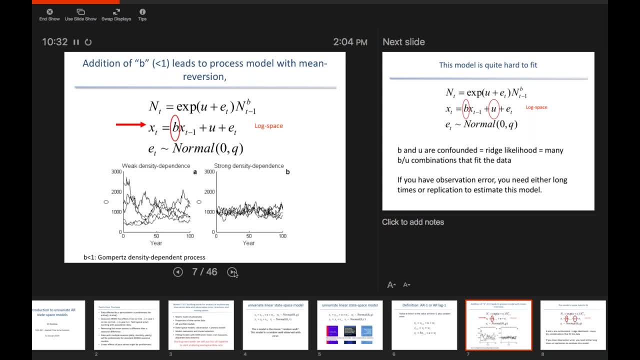 So here's an example. this is B is really close to one. if this was about, B is 0.85 and you can see that this process, and this is population size, is kind of wandering. It does have a level about a thousand, then it's minus one, so that's about a thousand. 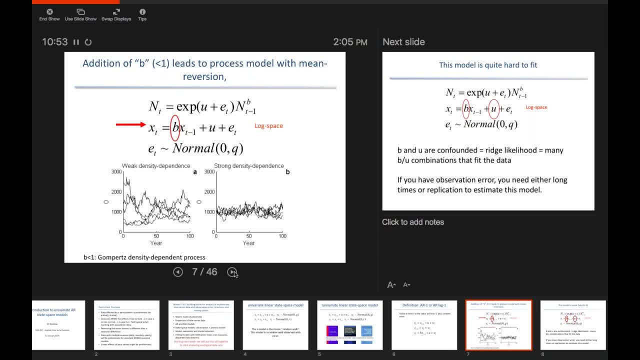 So it's about a thousand and then it's minus two. it's fluctuating around, but it fluctuates weakly around that and this one B is about. this is about 0.2 and you can see it's fluctuating very tightly. this type of model has been used a lot in studying marine ecosystems and 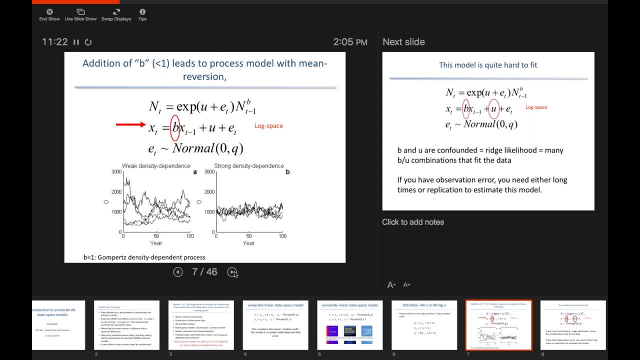 freshwater systems and looking at especially plankton dynamics- and I'll talk about that at the end- and using this class of model to try to understand how plankton species are interacting with each other. but the density dependent part of that- how that the species is infecting itself- is that 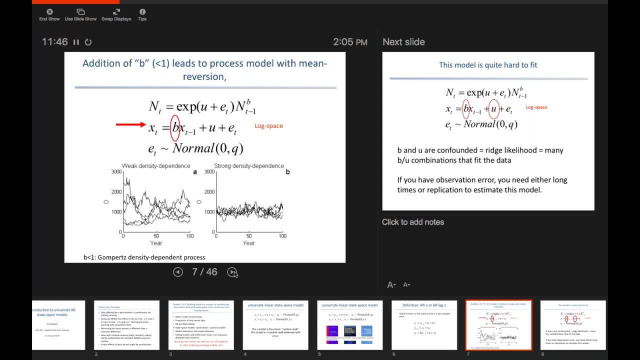 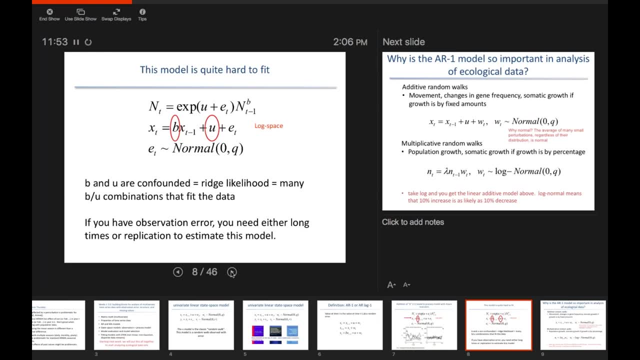 model right there. one thing to know about this class of model- which we're going to be using a lot, by the way- is that it can be hard to fit, and the reason that it can be hard to fit is that the B and the U parameters. so this is your strength of. 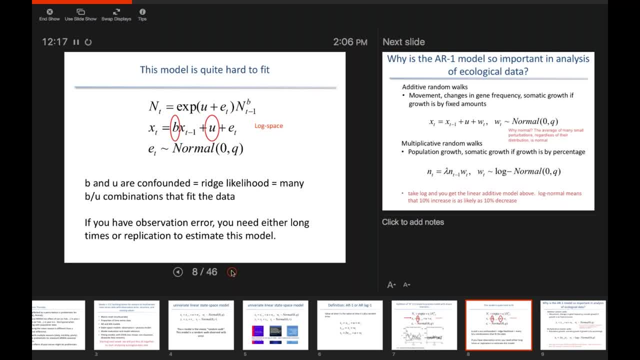 density dependence, and this is this parameter that is below the B and the U parameters, because the B and the U and the U are different. if you plot them that way, your B and U parameters are different and the H of the model say that the B is greater than or equal to the B and the U. 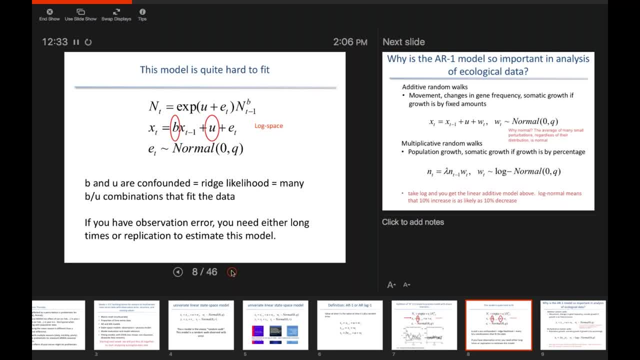 parameters. so this is what you're actually seeing, and using that model to kind of give you a way of understanding whether or not we're on the same track. it's only going to be a little different because it's a clear certification of that, because this is going to be a very interesting point to work with, the 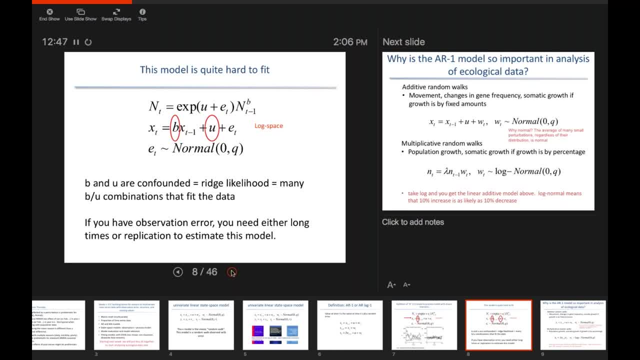 way that you're doing it, because it's going to be interesting to see how it's being used and then you're going to be able to practice it if you're already see that there's a peak, but there's also this big ridge in the likelihood surface. 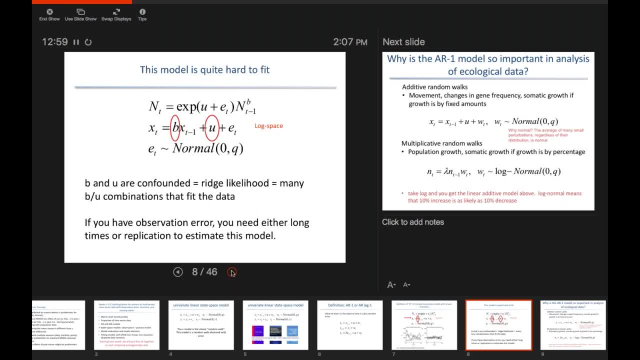 And whenever you have ridges in a likelihood surface when you have an algorithm, it doesn't matter what algorithm that you're using. it doesn't matter if it's Frequentist or it's Bayesian. when you have these ridges, the algorithm is going to get kind of lost on. 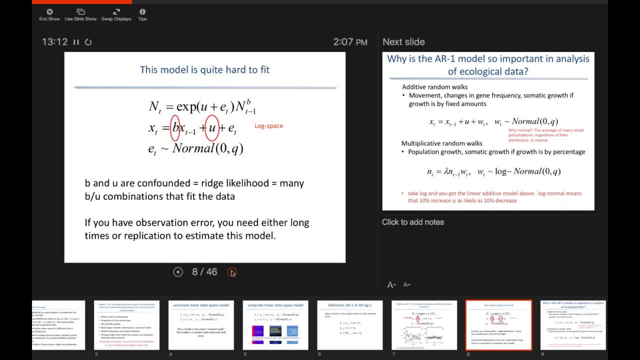 the ridge and it's really hard to find the peak and you need a lot of data. So, with this class, what we're going to be doing- you'll see the examples- we're going to be doing some tricks to get rid of that perimeter, so we don't have to deal with that. 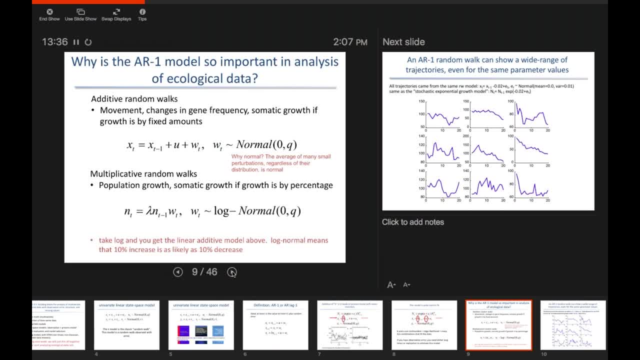 Okay, so I mentioned on Thursday that random walks are really important in the biological and ecological sciences, And so some of the Some of the problems where this class of model comes up is movement models set of gene frequency. Another example would be somatic growth, where the growth is by fixed amount. 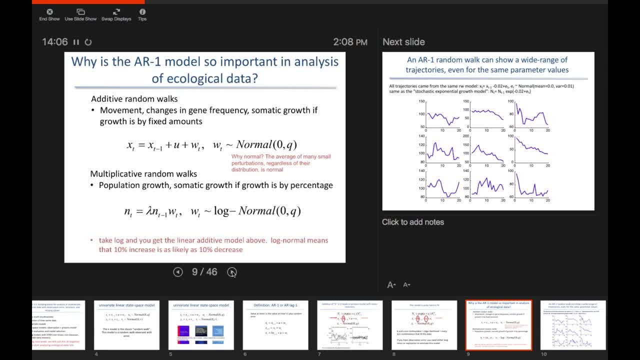 So that would be like an additive random walk. We can also have these multiplicative random walks that look like this: So it's a random walk because we have the n at time t is a function of n at t minus one, And this is going to come up. 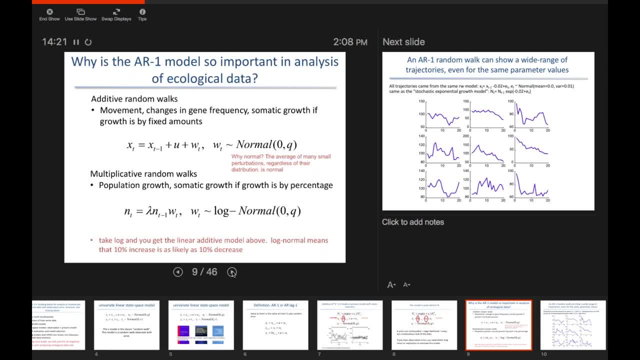 It's going to come up in population growth. So this right here would just be exponential growth. It also comes in somatic growth if the growth is by a percentage And if we take this model and we take the log of that, we come back to that model. 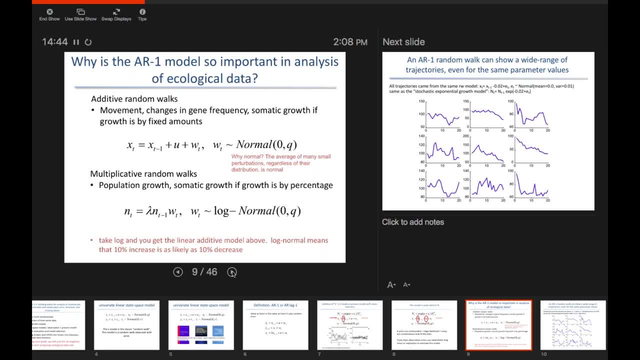 The errors in these models are classically assumed to be normal. Okay, You don't have to do that. Also, people will look at models where you have long tails and that can have some really interesting effects. You can have things like suddenly jump to a completely new value if you have these long. 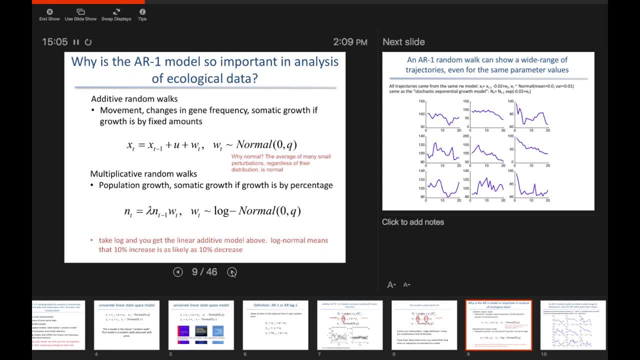 tails, But classically it's assumed to be normal And you can think about that as Let's think about population growth Right And the population size next year. It's affected by a whole bunch of little perturbations of what was the survival from. 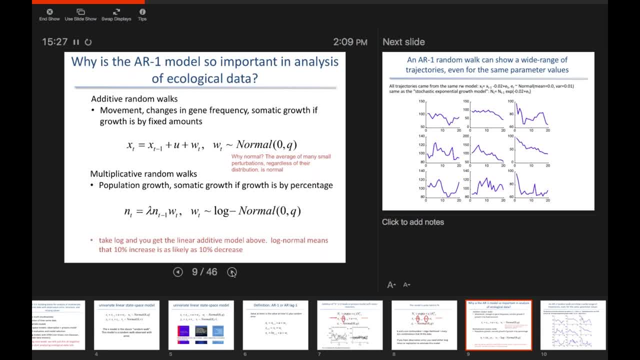 today to yesterday, Yesterday, Sorry, From yesterday to today, Today to tomorrow. It's all of these little bitty perturbations, And if you take the average of a whole bunch of little perturbations, you're going to come up with something that's normal. 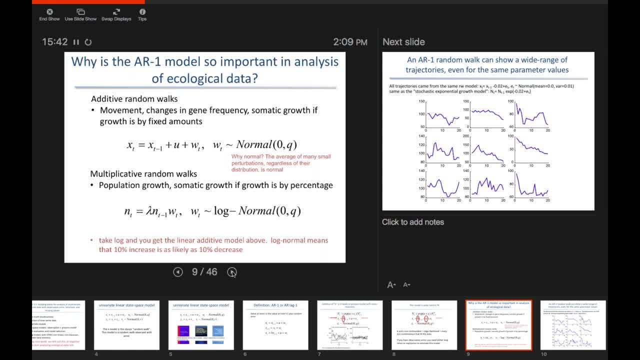 So that's kind of the sort of back of the envelope reason why we often see: well, it's going to be normal, Right, So why we assume normality. But also, if you look at the differences, you estimate these models. we look at the differences. 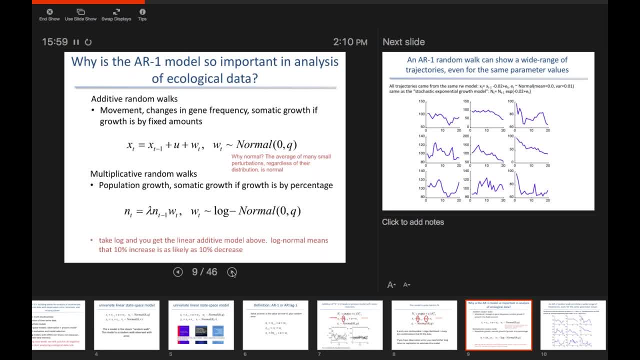 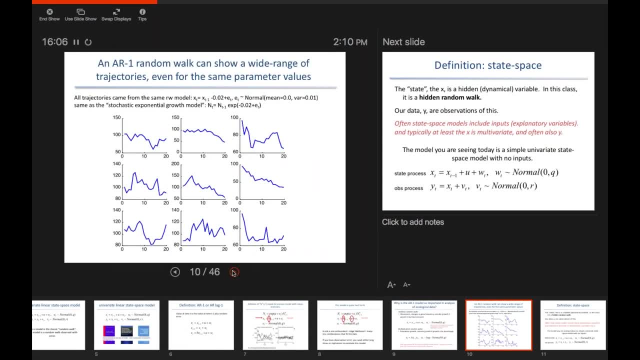 that you often see the errors. look about normal. So here's a plot of a whole bunch of different random walks. Okay, And the thing to note about this is that these were all simulated with exactly the same parameter values And it was, on average, a slight decline and the variance was pretty small. 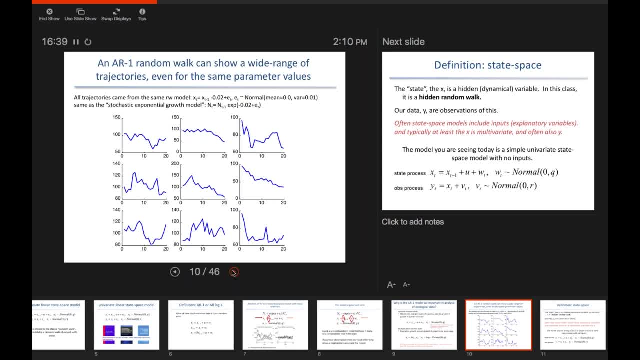 It's not really big variance. This is pretty typical if you were to fit a model like this to some population data. So it's pretty similar to the variance that you would estimate. Okay, The variance that you would estimate Something quite small. 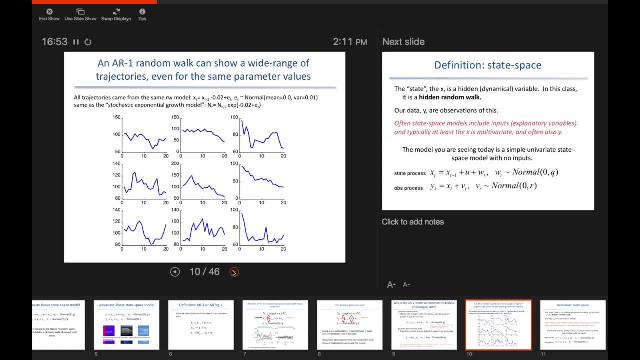 The variance of .01.. And so you can see that with the same parameter values you can get very different trajectories. And I point that out because you know, when we look at data, we have this And we look at that and we're like, wow, this is really different. 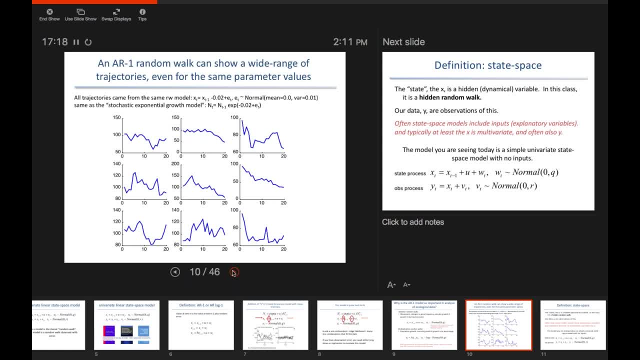 Let's look at this data. Okay, like wow, something, something really different happened, perhaps like my whole system changed here and when you. you should recognize, however, that if you're fitting up with a random walk, that's not necessarily the case that your system is the the sort of the underlying structure of the model is to be very 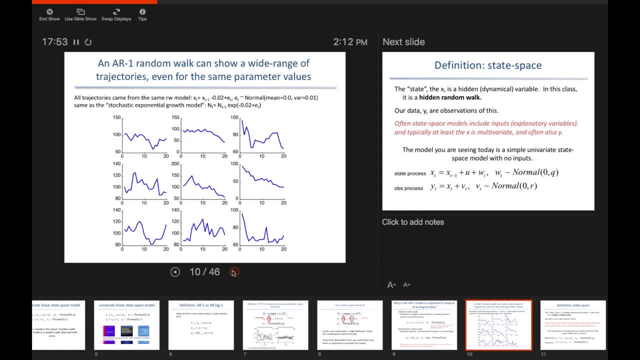 very much. what could be exactly the same for this versus this? and the only thing that's different is it just so happened that the error terms were: it must have been negative here for the few few concepts, right, and then the positive result back up, but the structure of the model is. 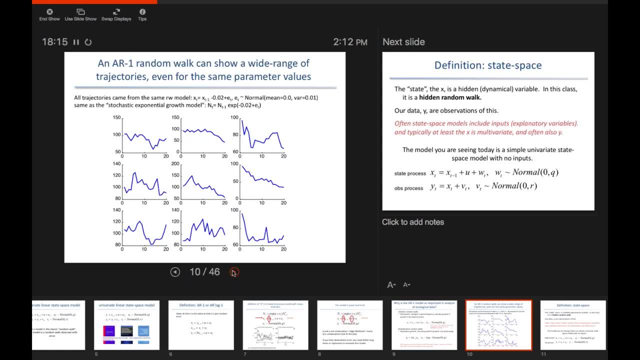 exactly the same as the model, but the structure of the model is exactly the same. the parameters are exactly the same. this is- we're going to run into this- when we start working with real data and we quantify our uncertainty. so if you look at that, you should have this sense of like: oh yeah, there's probably you. 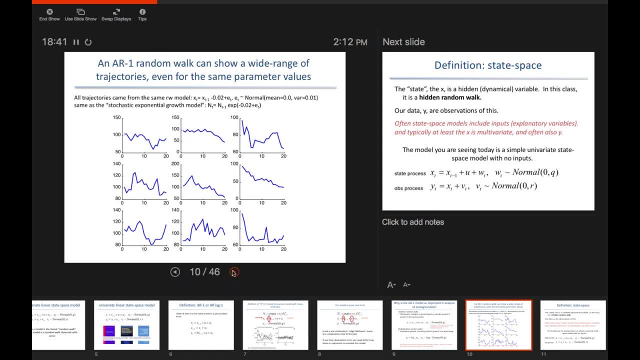 know if one set of parameters can produce all of that, then so you know another set of parameters that can produce all of that, then you know, probably would get that happening then. so this just kind of a conseguent error, or this an error or something, but a set of parameters, that's just. 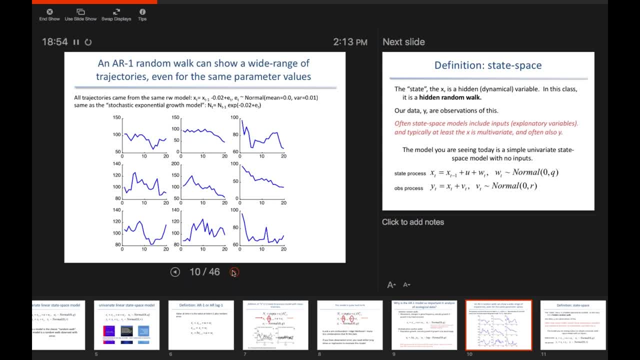 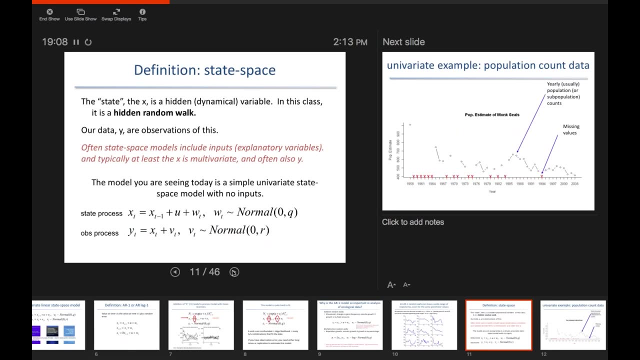 slightly different, could also have produced all these or something that looks kind of similar to this, and so you shouldn't surprise you when we started when we show you the uncertainty about our parameter estimates that they're going to be pretty right. often I'm going to need a lot of data to 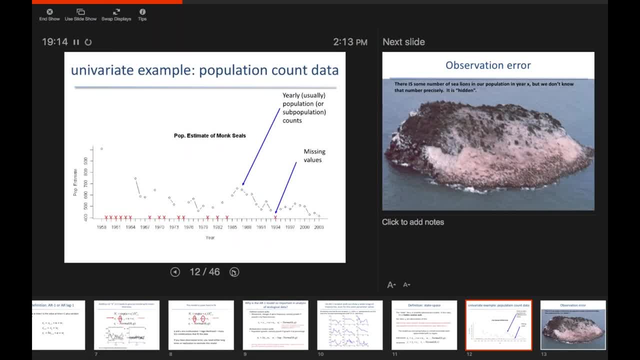 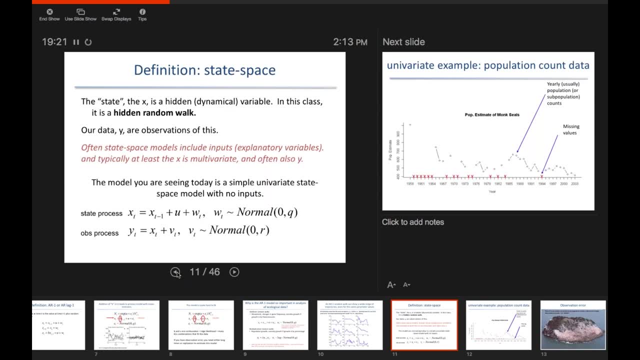 estimate. some of these partners Talked about that, So let's see some examples of let's go back here. Okay, so I've been talking about the state process. Now we're going to jump. we're going to talk about the observation process, And this is something that makes 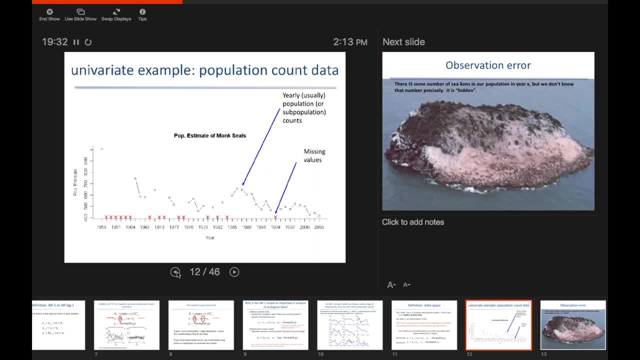 working with ecological data really hard. It's kind of unique to us relative to other areas of science where we can do an experiment and we can understand in great detail our observation error process. For example, we can repeat our experiment over and over. If we have a temperature gauge, we can stick that. 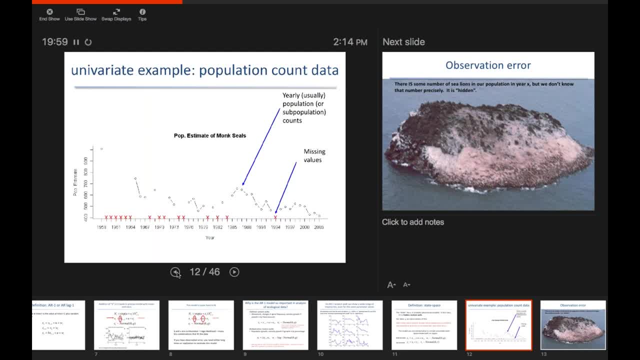 temperature gauge in a known temperature and know what the error rate of that temperature gauge is. But when we're working with ecological data, fisheries data, we don't. we often are not able to know exactly what our observation errors are. Okay, so here's an example. This happens between monk seals And then 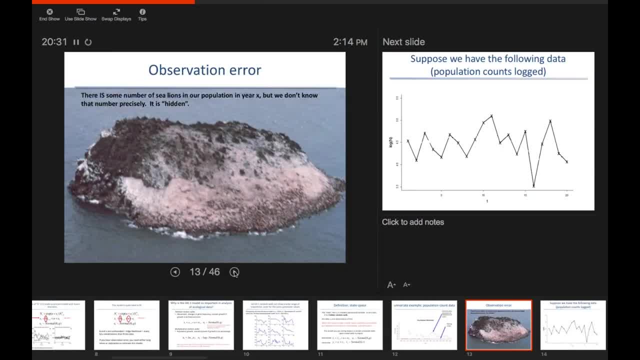 here. I want to show you another example. This is what I wanted to show. So this is this is an example of a fine example of observation error in real data. This is a actual survey photograph for stellar sea lions. I worked for many years on steller sea. 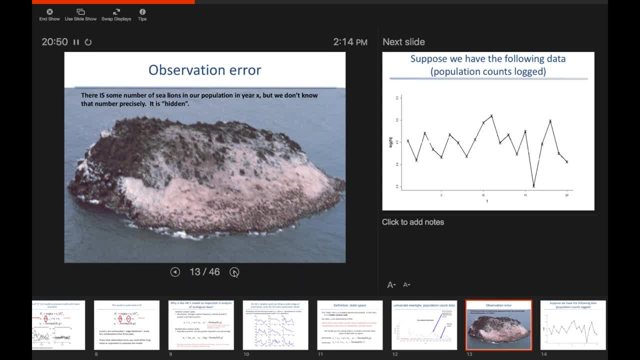 lions. and this: this is a real photograph taken from an airplane. And now we're going to go and we're going to count all the stellar sea lions here. So you can see, obviously we're going to have a total of signatures. They're not. 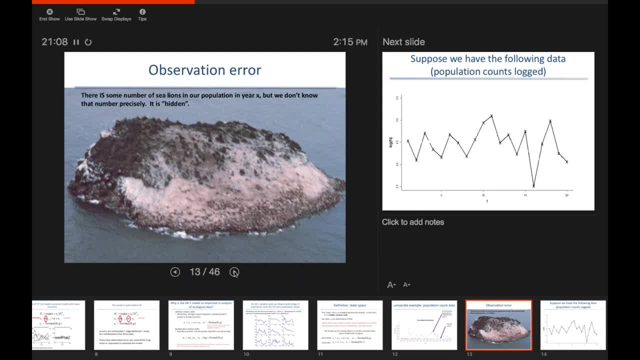 으니까 engandere sarai tar chef sirago asessio. we're needles andêmes La have. observation error, And it's not just the fact that this is a photograph and it's fuzzy and the sea lions are kind of half on top of each other. we got. 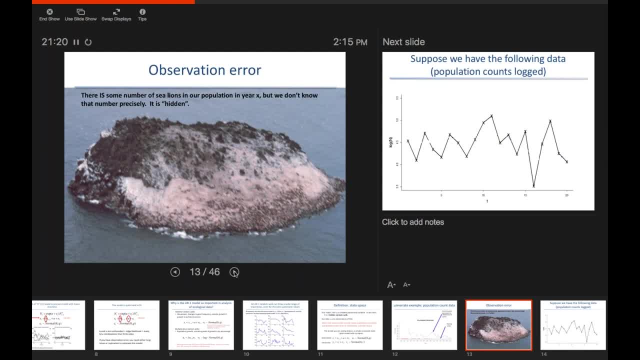 that problem. But we also have a problem that there's sea lions on the other side of that island that we don't see, And there are sea lions in the water and we don't see them either. Right, so we have all these different sources of. 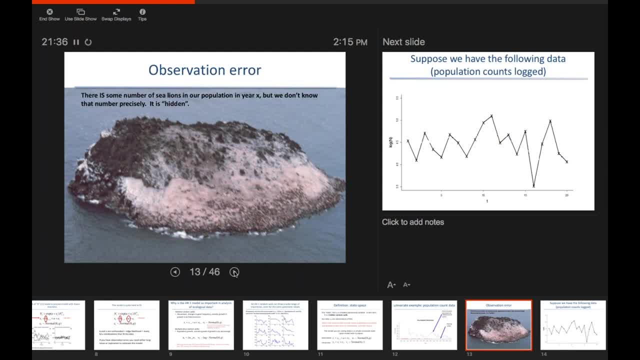 observation error and we don't understand, we're not going to be able to understand the magnitude of these and how they're changing with the, how our environment is changing Right. so, for example, we have sea lions in the water. What is driving them into the water Food? So we have some. 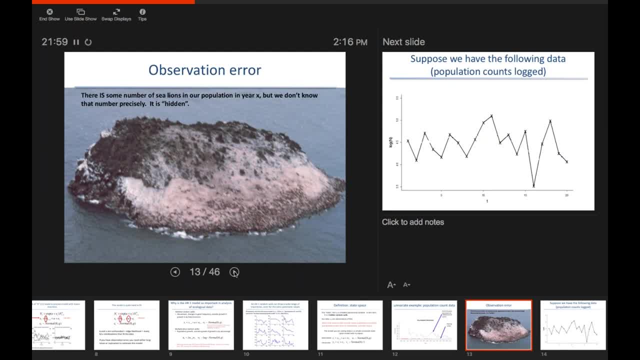 variability in the food that they're going out to forage for. We don't know. you know how close that food source is to this island. If that food source is very close, they don't have to spend a lot of time in the water. If it's farther away, they. 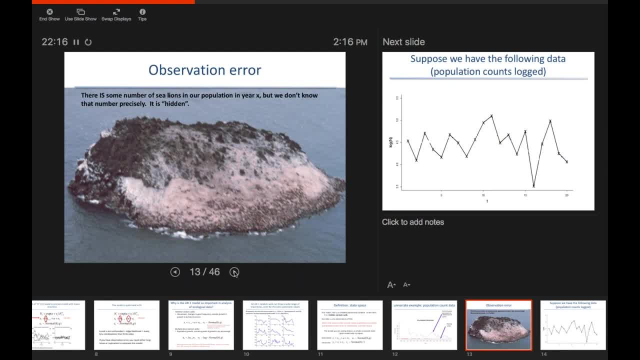 spend more time in the water, so there's fewer than one island, So we have those kind of things. They're adding all this variability to our data And we can go out and we can do things to understand how understand how to study sea lions, And we can go out and we can do things to understand how understand how. 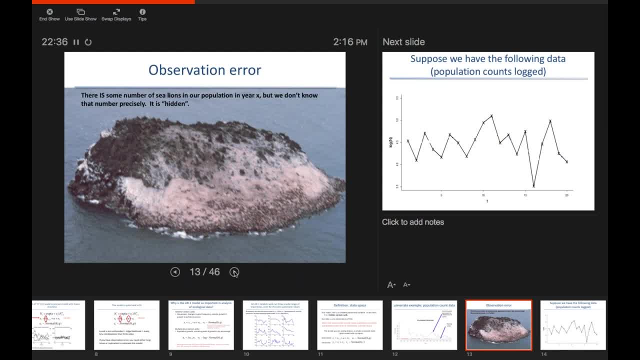 understand our survey variability right. so imagine, instead of having a survey like this, imagine that we have a ship survey and we're going out and you know we can think about experiments that we might do to understand what our standard error of our population estimate is, our survey estimate is. but there's going to. 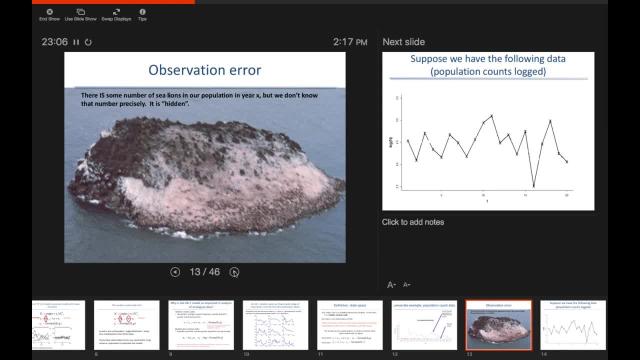 be all these other things that affect citability. we're not going to be able to do an experiment, so it's just like, fundamentally, that it's different for us that we have to estimate the observation error of variance. we just are not going to know fully what that variance is and all the different components, okay, so 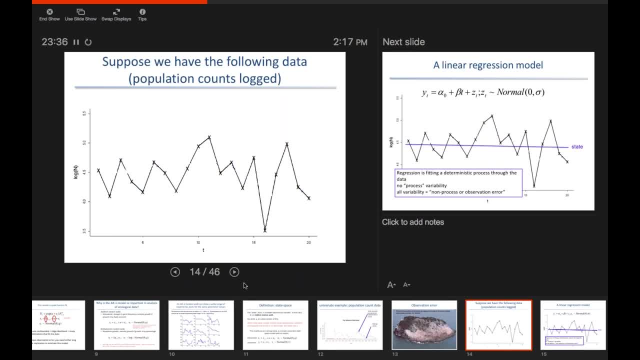 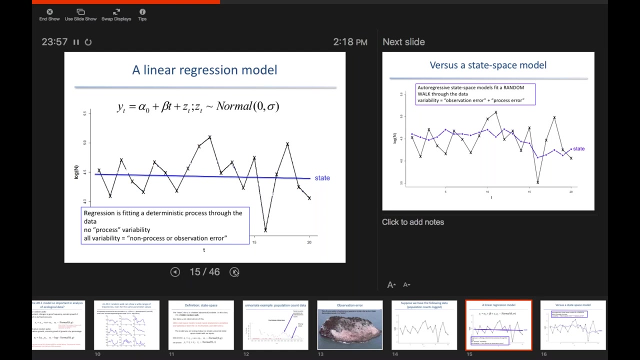 let's see some examples with some data and let's start getting a better sense, mathematically, what observation error is. so let's say that these are our population counts. you have 20 of them and now we're going to fit a model. so we're going to start by fitting a linear regression model. that model is we can say: 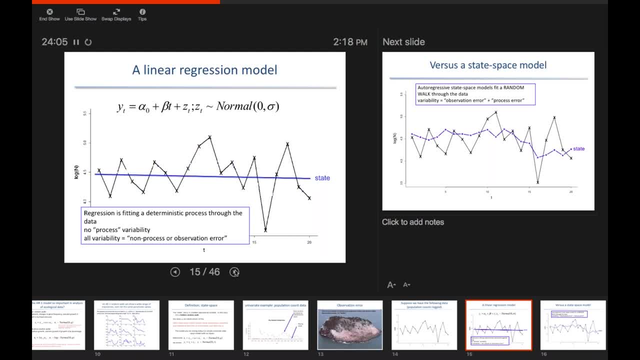 frame that as a state space model. but what we're going to say is that our state is the straight line and now our data are: this part here, this is our state, and our data Y are our state. right there it's deterministic plus some error. so I've written this just as one equation, but you can think of this as to. 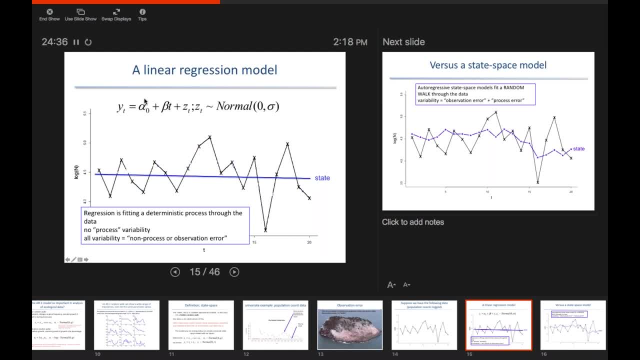 XT equals alpha 0 plus beta T and then YT. is that XT plus this error and our observation errors then, are the difference between the state and the observation? this sort of model where you just fit a linear regression that would be. that's actually, you know, a common thing to do, if you think about, if you have a 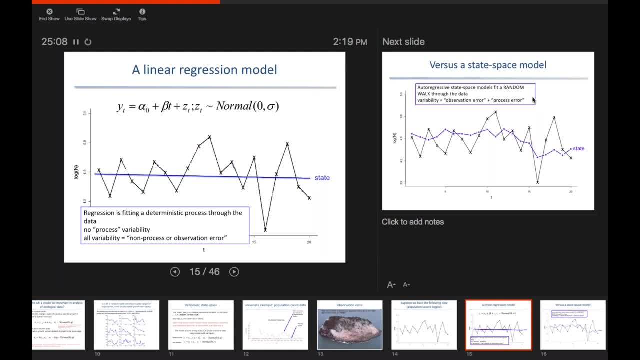 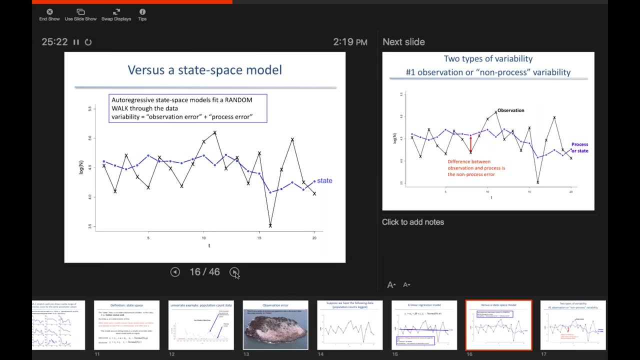 population count data. you want to know what the trends are. you just put a linear regression to it and then you get the average trend. in this case, it's about the trend of zero. it's not increasing or decreasing. and then when we have the random walk model, we have this. now we have that. that state is not. 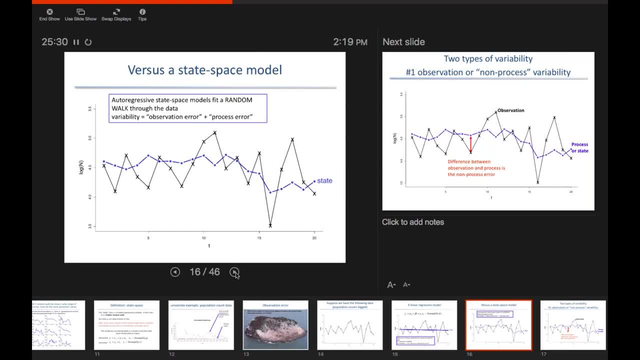 a straight line, but rather it's a random walk. so this is what we- and again, the observation error is the difference between this and this. yeah, yeah, so that you've got it's xT equals X t minus one plus the u. that's a random walk. and then, if you have a random walk, you're xt-less. so I'm going to figure this out. And then you sum that up and then you connect the random walk of Paris. So I'm beginning to figure this out. Then I think we're going to have a good view of the curve here, So I'm going to go back to last part of the picture. So I'm going to go back to the graph here and I'm going to go through the graph and then I'm going to go over this graph here. Then I'm going to go back to the graph here and I'm going to go over this graph here. 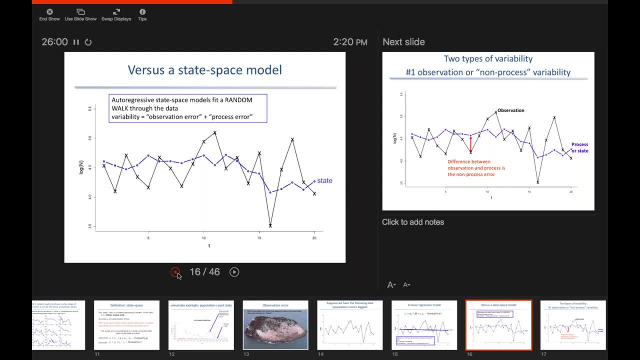 trend. so you got that one, and then you also need to estimate that variance. so how we believe is this? that's going to be determined by the process where grants, and then for your observation, you have your observation variance, which is: how big do these errors tend to be right, okay, so you're going to have the 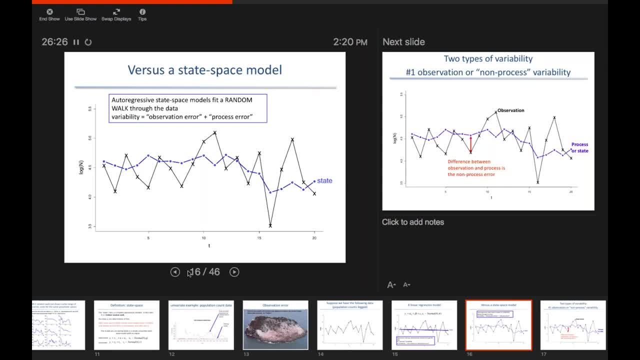 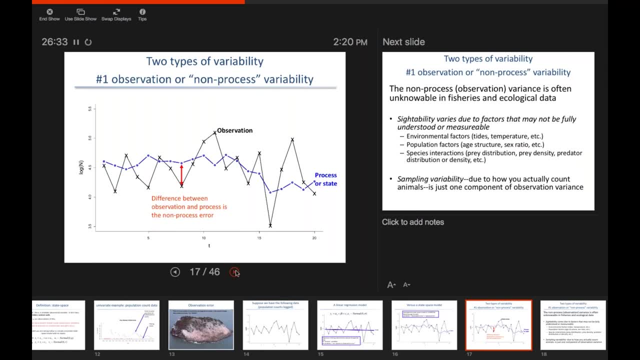 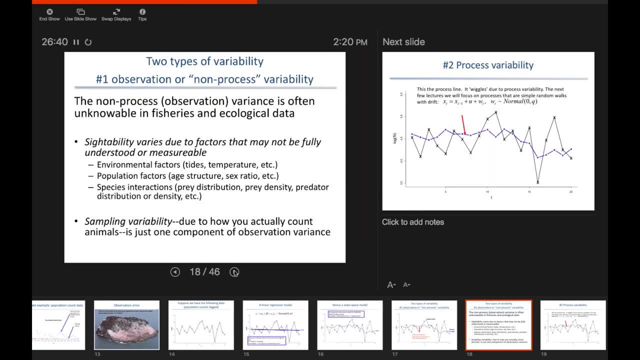 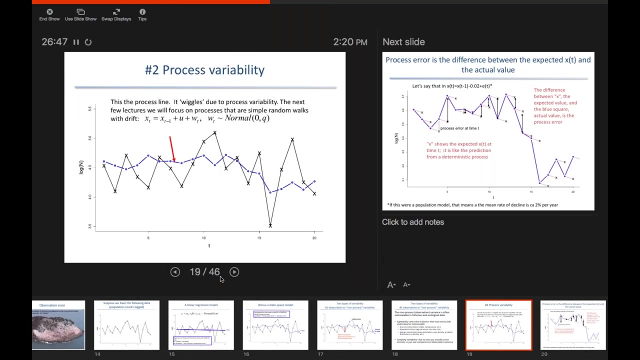 simplest version. you're going to have three parameters to estimate. we're going to do that in just a few minutes, okay, so I already talked about this. these are the issues with citability, why we need to estimate those two variances. okay, talk about a process variance, okay. 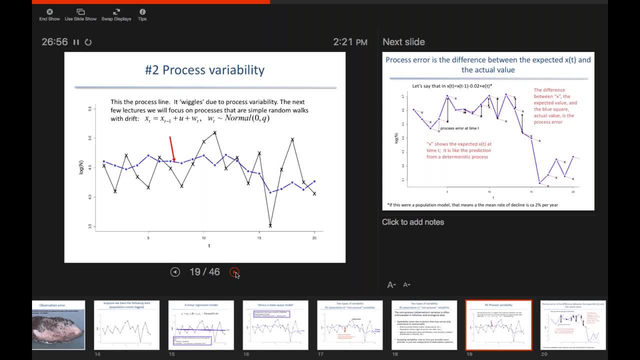 so the observation variance is pretty simple to wrap your head around. it's just the difference between your estimated state and or the. it's actually the difference between the true state and the observation. we're going to estimate this, but you can imagine that you know there exists some state. we just 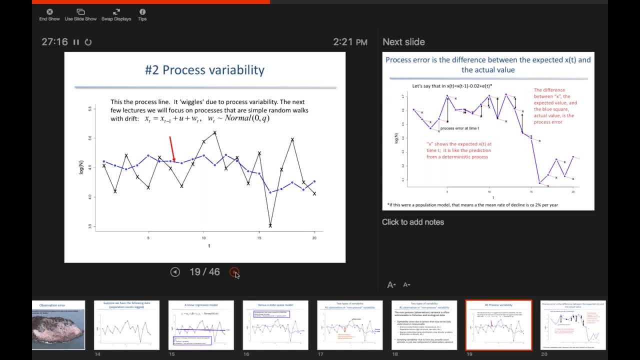 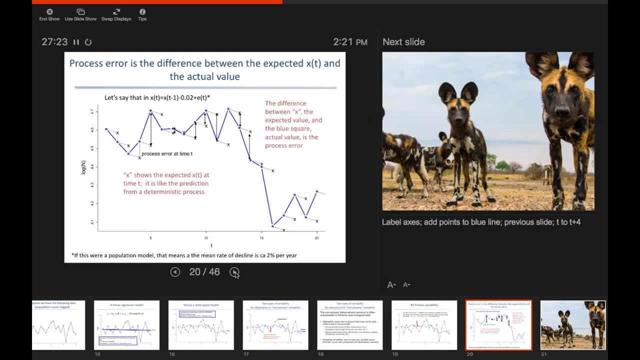 don't know what. it is okay, so that that's your observation error. the process error is this. so here's, this is just the state. okay, the blue is that hidden state. let's think of this as population size. this is the actual population size is the blue. 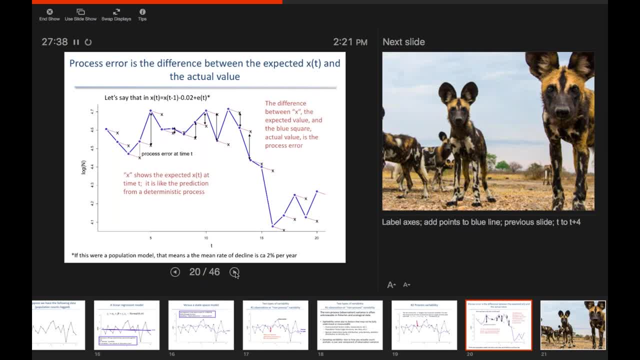 line. we don't observe this. we observe this with error, don't observe the truth, the process. error is the difference between what you would predict about. the population size has to be given your value today. so what do you predict it will be tomorrow, and that prediction is based on the trend trend estimate. so 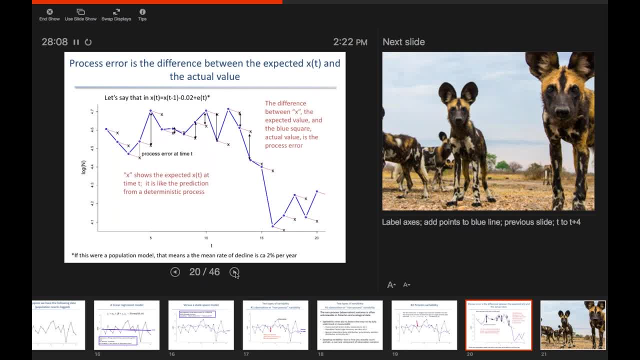 here is a negative 0.02, so it's estimating that it goes down 2%. predict it will be here, but then actually it was here. so the difference between what you predict it would be and what it actually ends up being, those are the process errors. if that process error variance is very large, this will be. 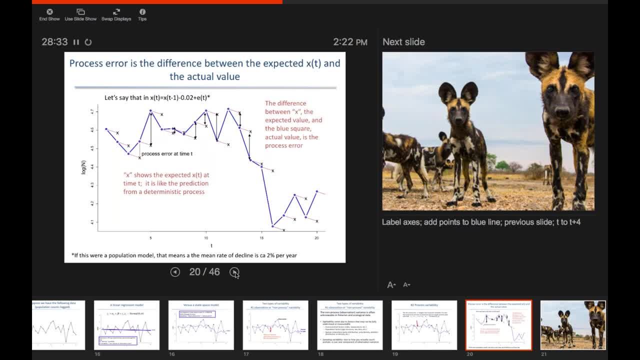 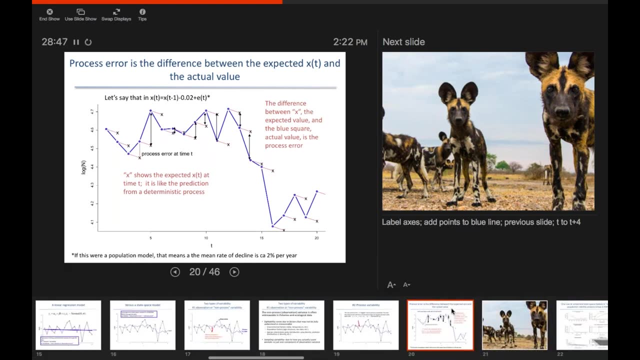 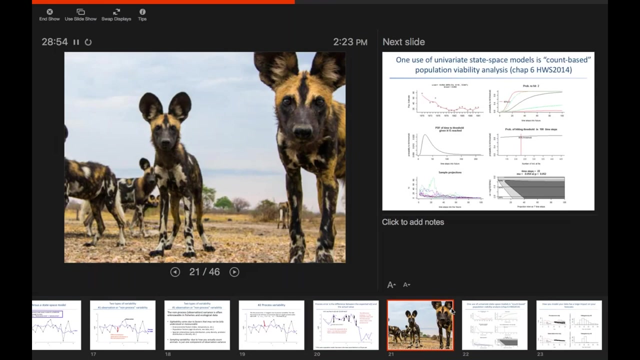 very wiggly and tend to very quickly wander off. if this is very, if that process variance is very small, it'll just tend to go up and down, okay, okay. so let's see this in action, how you actually use this. I'm going to show an example of doing a population viability analysis for wild dogs in. 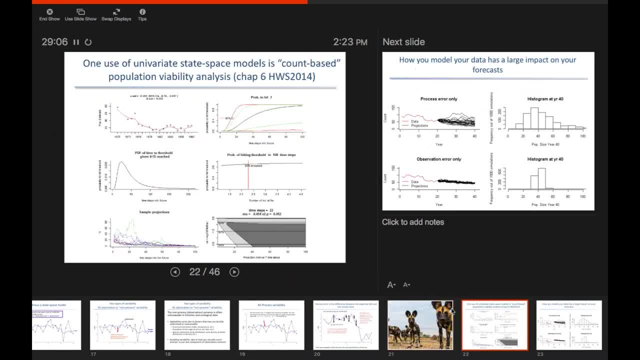 Africa are critically endangered. this is example of what's called a pelt based population viability analysis. and what do you want to do? want to fit to those data points? The data points are the wild dog counts between 1970 and 1991, and those counts have error. so we want to estimate what the 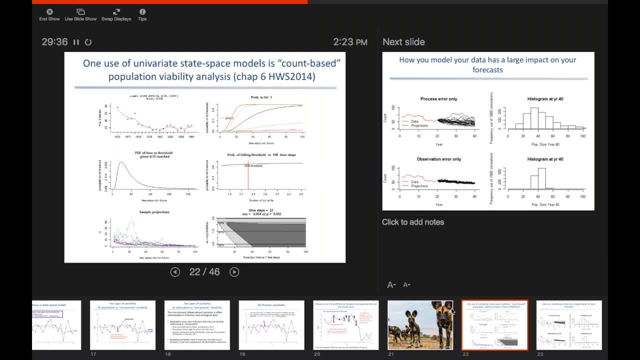 true population size was the red line and from that we want to get the U estimate, which is our trend. Remember it's xt, xt equals xt minus one plus the U, plus the error terms, and that U is, on average, how much it's going down or how. 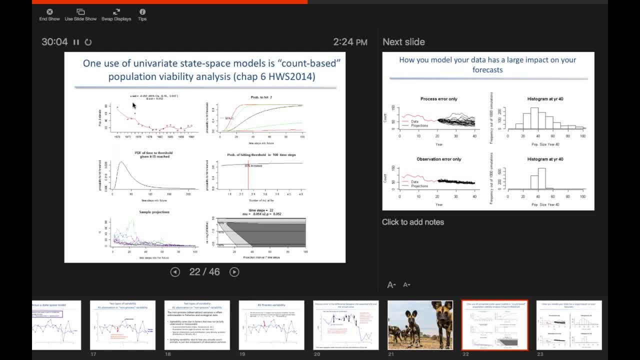 much. it's going up and so this is negative zero point five point zero. sorry, negative point zero five four. That's a very steep decline. and then here's some samples, projections using that and using the estimated process variance. so I'm just 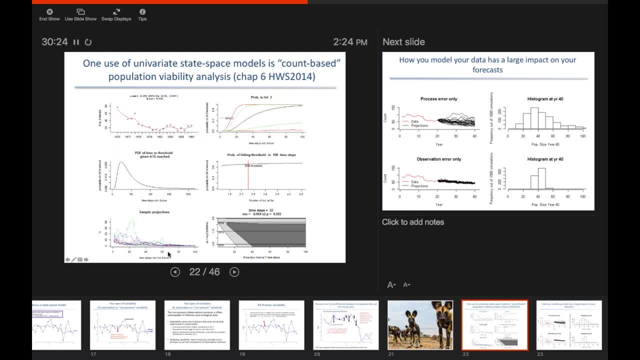 simulating the red line and you can see it's all going down to zero here. and then what you can do, once you have those estimates, is you can compute things like what's the probability of hitting a population size of two and at certain 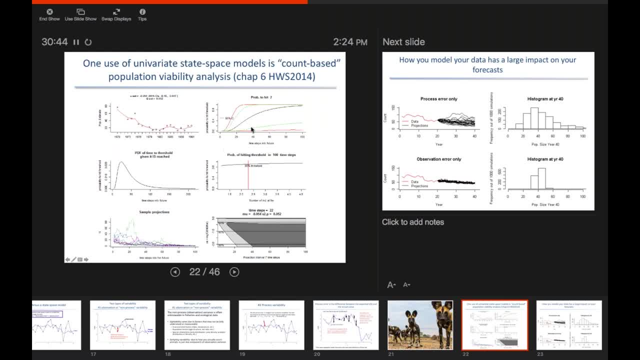 times of the future. this is the average. so what this is saying is that at 50 years in the future, there's a very high probability- about 50%- that it will hit threshold- a population size of two. And then you can also portray your uncertainty by looking at. this is in the 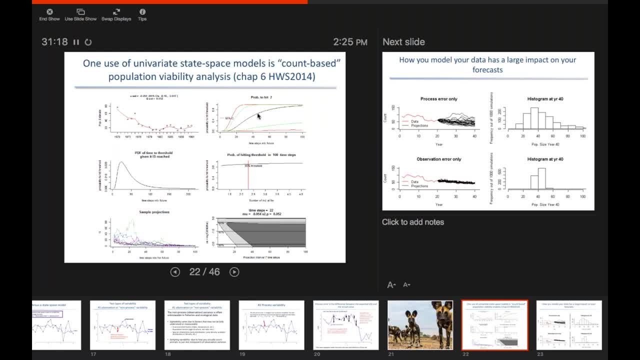 future and this is the population size. so this would be a 50% decline, 90% decline, 99% decline and what you could say is: this dark area is very certain. this is highly uncertain. this is who knows. so you can see there's a lot of uncertainty there. 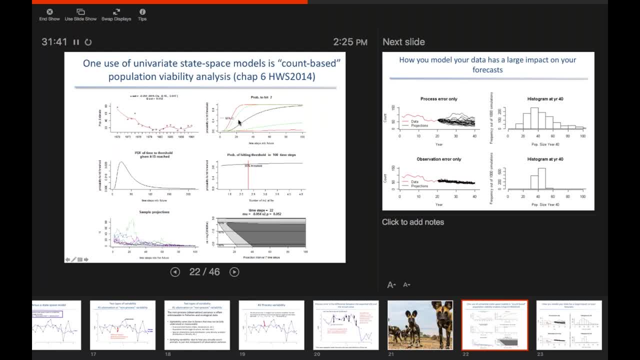 the green line is your, I think that's 80%, and the red line is to the 95% confidence intervals. so you can see already here it's like who knows what's happening in 40 years. it's 0 to 1 that we would hit a population size of 2. so 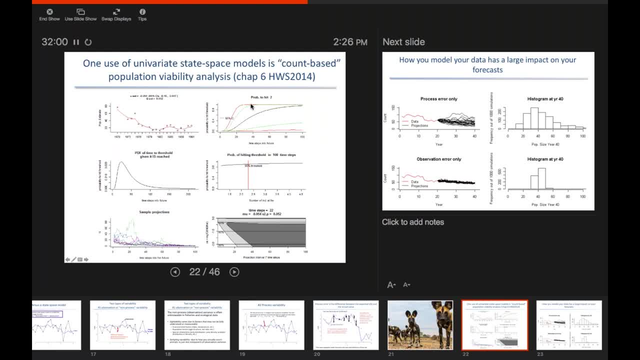 it's saying: you know it could be a 0% chance or it could be a hundred percent chance. but then you can take a whole bunch of plots that look like this and you can see this was a 99% decline order, that somewhere at that point is. 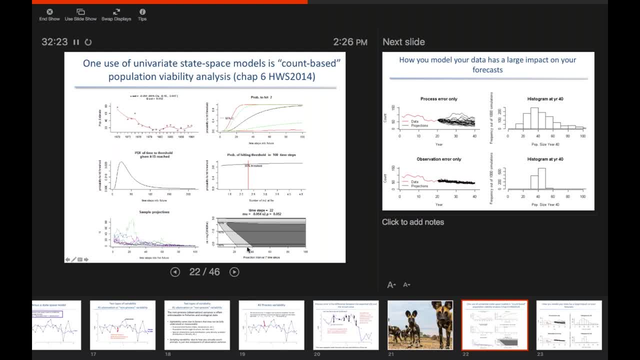 somewhere right around here, and what that's saying is that we're really uncertain about projections that are you know about. you know we're not sure what's going on with the population size, but we're concerned about it and we're going to see what happens in the future. 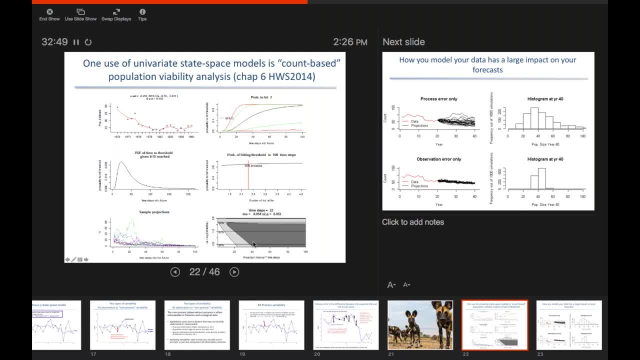 again. we'll do this. we've got so here: 0 to 1. we've got 0 to 1. I can look at this carefully enough before I record the lecture. But basically what you can do is you can map out these regions where you are very certain. 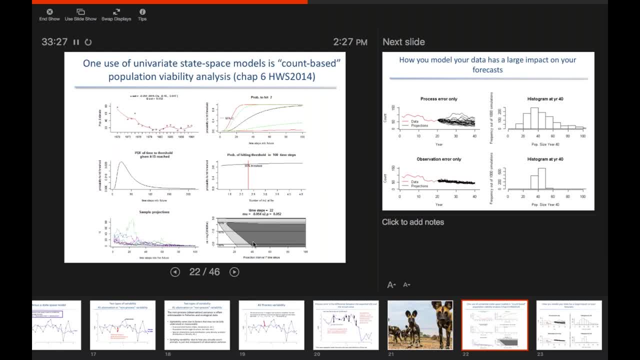 about what's going to happen, and then regions where you're uncertain. So even though you might have a plot like that, where there are parts where you're very uncertain, very uncertain, out here, you could be quite certain that nothing all that terrible is going to happen in the next, or you're not likely to hit a threshold of two in the 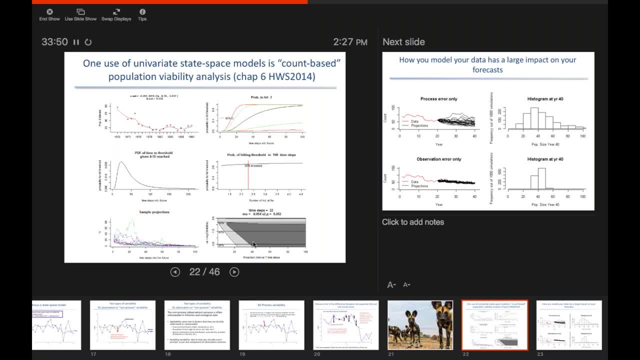 next, say, five years? I can't remember what this is. So this is the uncertain region. So you're very uncertain about things that are very far in the future, but you're quite certain about things, Things that are closer, And you can quantify exactly when your uncertainty starts going up. 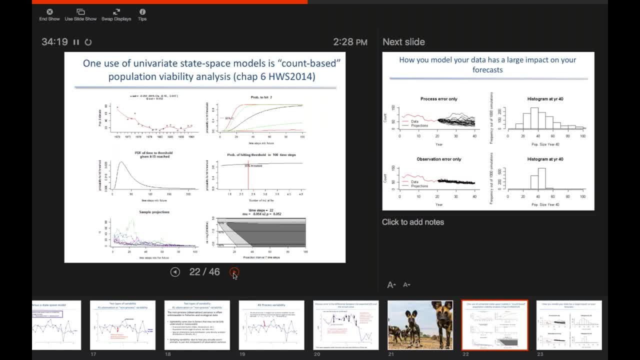 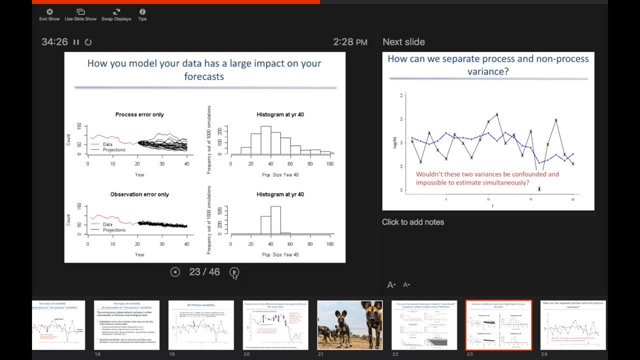 Okay, So why is it really important to separate these process errors and observation errors? Okay, So why is it really important to separate the variances and get a really good handle on what the size of these are? Well, the big reason is that it makes a really big difference in your projections if you 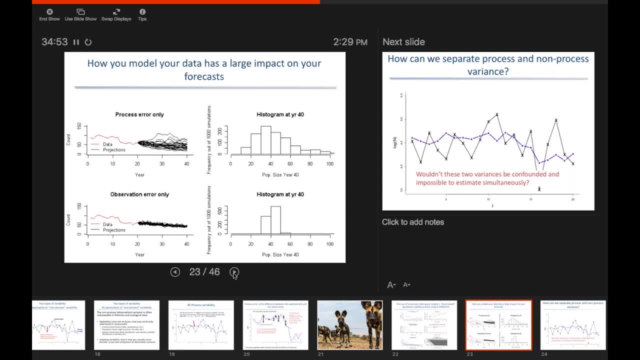 assume a model with only process error or only observation error. This observation error only is your linear regression. Okay, So this would be a typical Projection that you're going to do. if you just did a linear regression through this data, Did that? 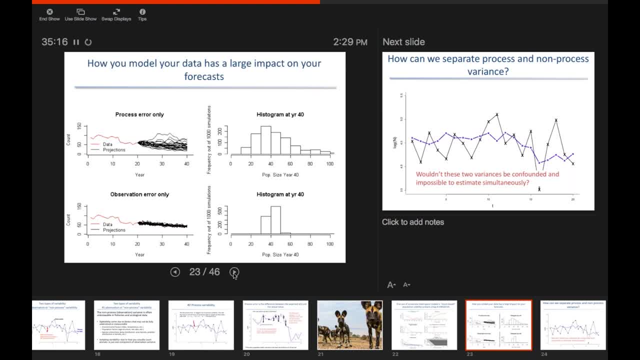 Okay, That's the trend. And then someone says, okay, well, what's the probability of hitting two out in the future? Are you going to forecast and you're going to say, well, that's very unlikely, This is what you would estimate. 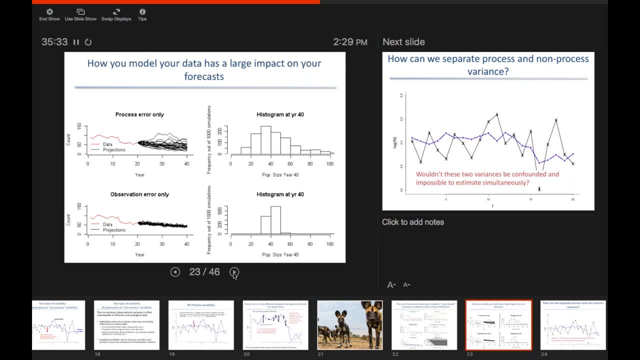 We've seen what we are simulating: random walks. Okay, They tend to explode. And here what we've done is fit a model that's only process error but mixed in the observation error with it. So I said, okay, yeah, I know that it's a random walk. 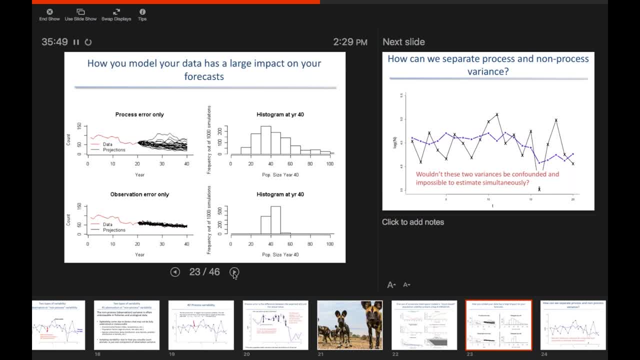 I know it's a population process. I'm just going to ignore that. there's any observation error, because I don't know what it is And I'm just going to ignore that. If I were to do that, I would. Okay, I'm just going to ignore that. 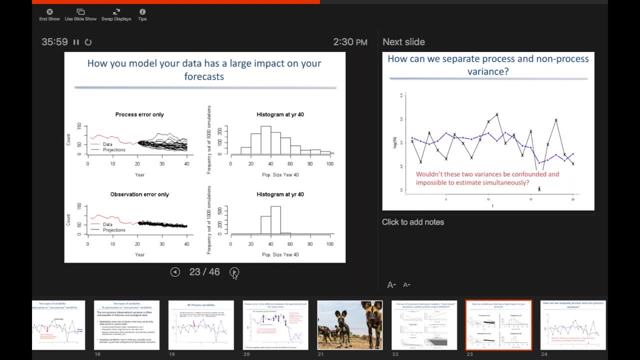 If I were to do that, I would: Okay, I'm just going to ignore that. I'm just going to ignore that. Okay, I'm just going to ignore that. I would estimate that the probability of hitting low values threshold is much, much. 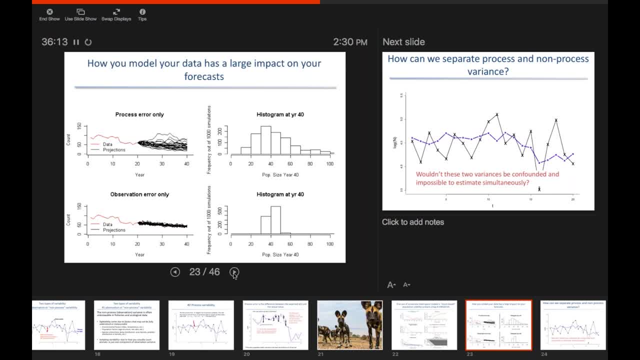 higher. The truth is somewhere right, Somewhere between these two, because the data half of process error, that is, the population size, does fluctuate from year to year. We know that. But we also know that there's some observation error. 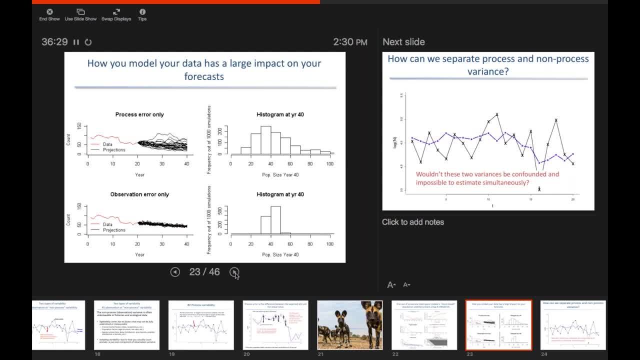 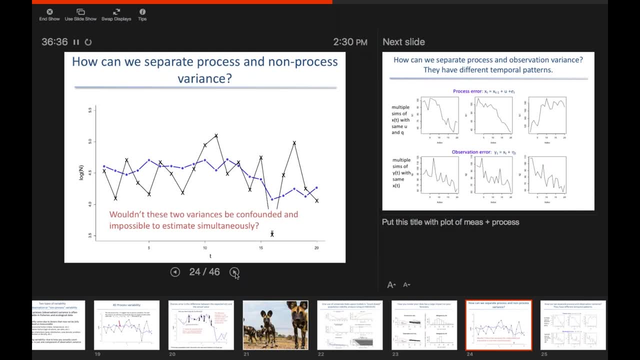 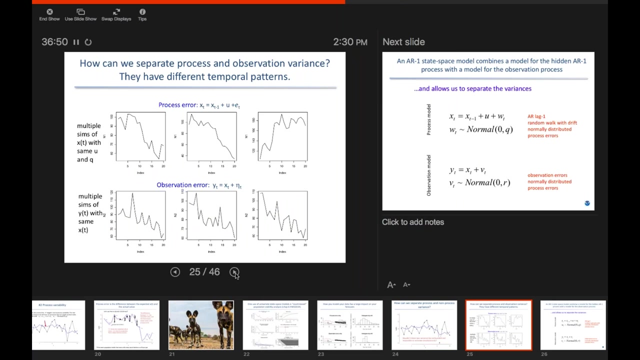 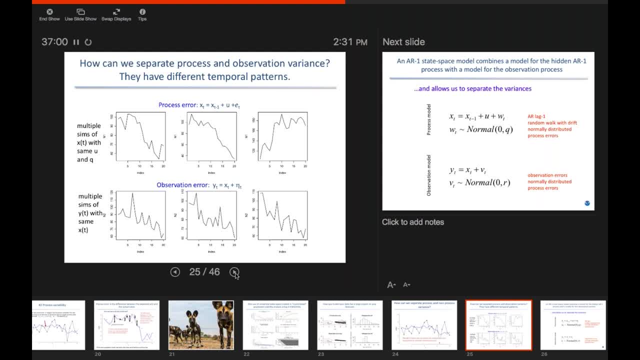 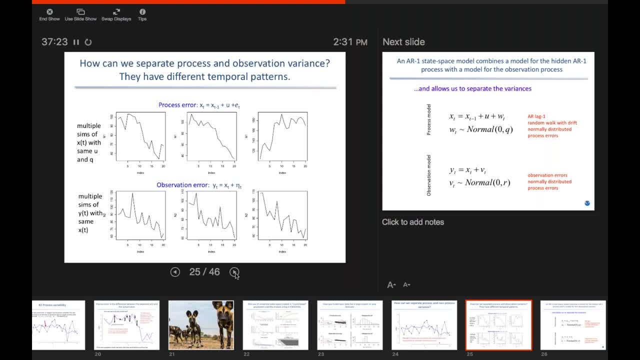 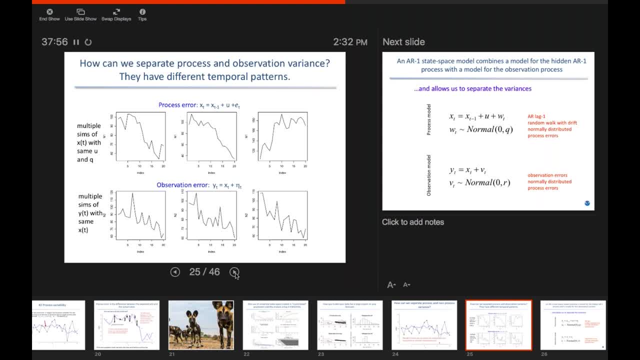 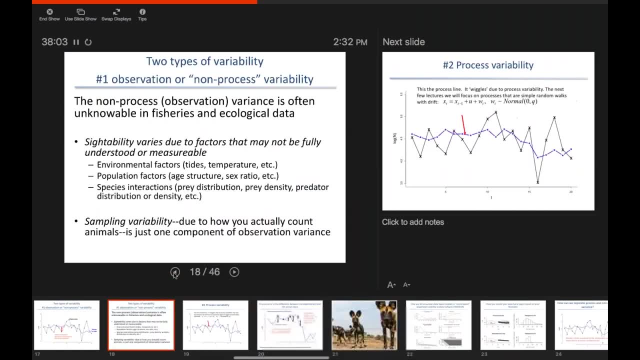 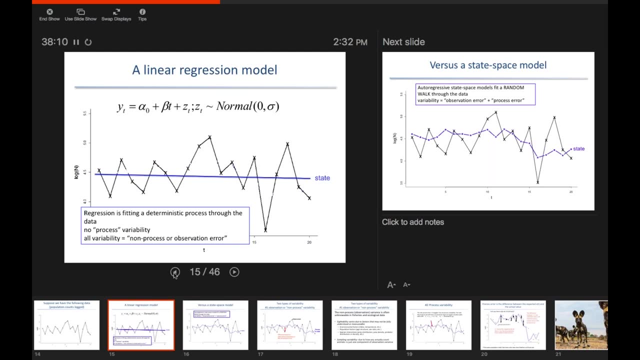 straight line to the data. all observation error, that's it. we would only get observation here and the other one. you would have a random block that just mapped on to the X's. exactly. so right, that's so. that's observation error only. and if we took away all the observation error and made all process, 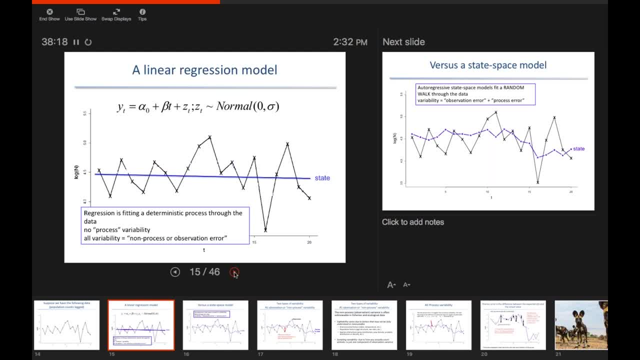 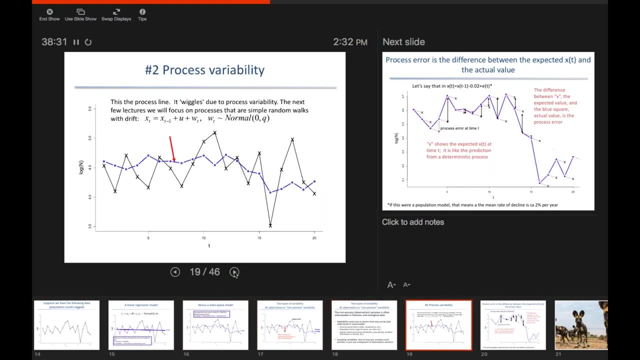 error. blue dots would be right on top of all the X's. so the algorithm is going to decide: okay, is it all one, all the other or a mix, and oftentimes it's a mix. that's the better, not always it's. we do things in lab, you know I doubt that sometimes you're. 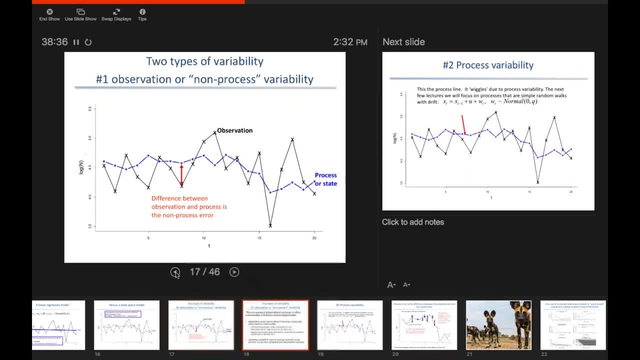 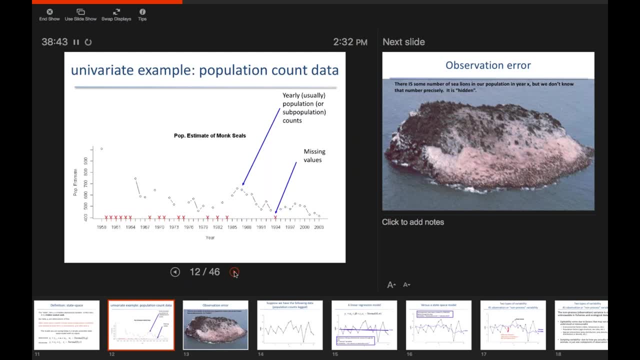 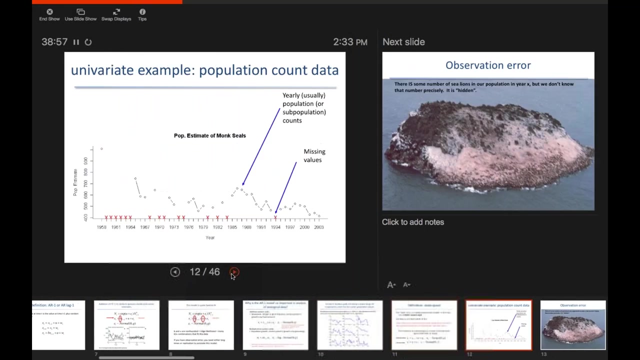 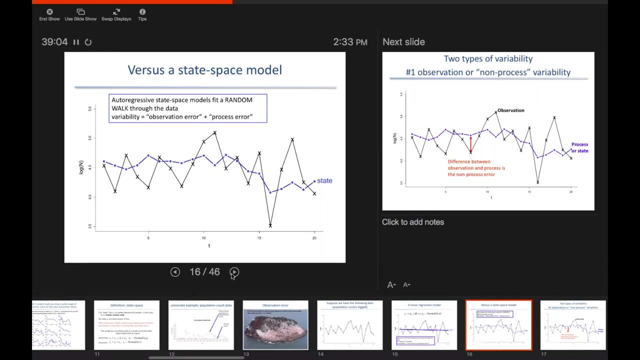 asking it to fit both, it will say, based on all the information you give me, is only observation error, it's only process error. and I mean you can think about mathematically. you look at those equations, you can write that right, the likelihood of the model. right, you can write the likelihood of that. and then you could write the. 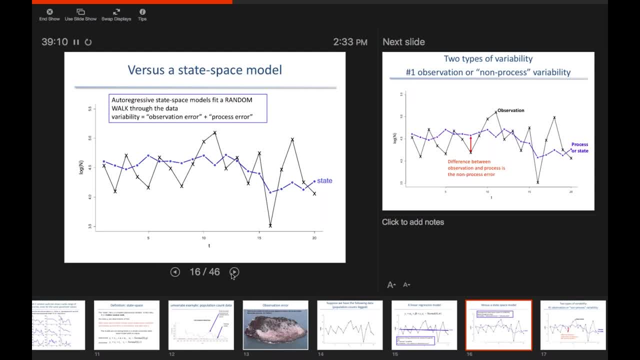 likelihood of making this blue line be the black line. so those would be the two extremes and then you write the likelihood of the model that includes both, that you're going to maximize that. but the reason that those variances are parameters, aren't completely confounded is that those two models, the random walk. 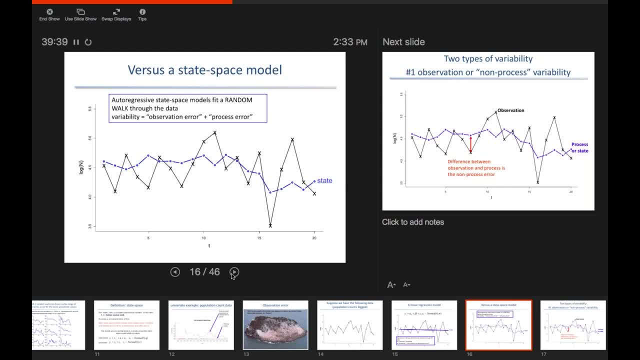 model and the observation only model. they have different temporal patterns. They're not. when you just simulate it out, you can see they look really different. If they didn't, if they looked pretty much the same, then you would be hopeless. 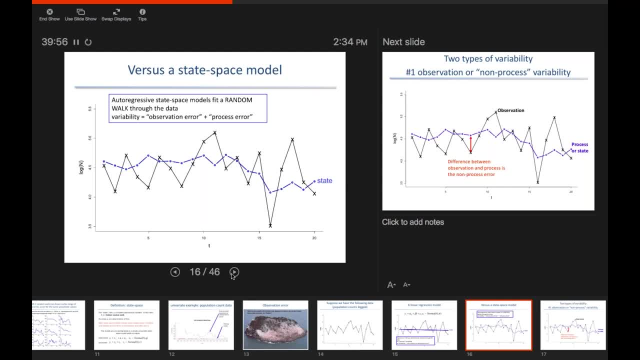 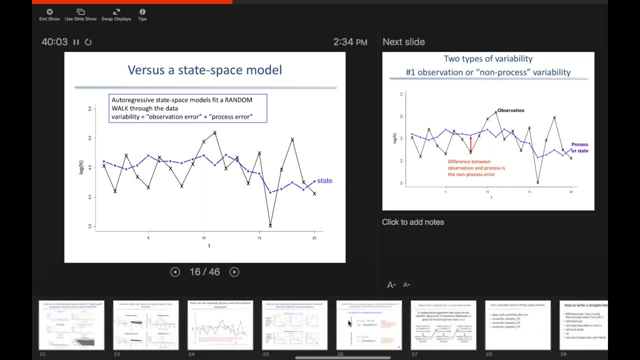 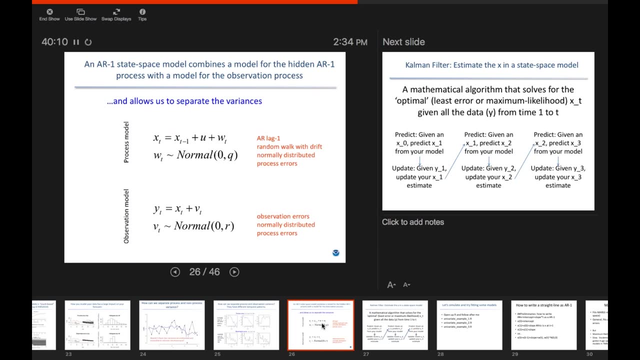 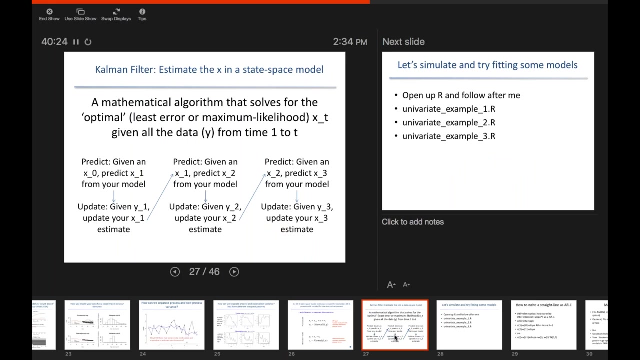 You'd never be able to separate things. because you're trying to, you know you're using models that can produce exactly the same kind of data. Okay, two more slides and then we're going to jump in and start doing this. Okay, so I want to briefly go over the Kalman filter, because you're going to hear this. 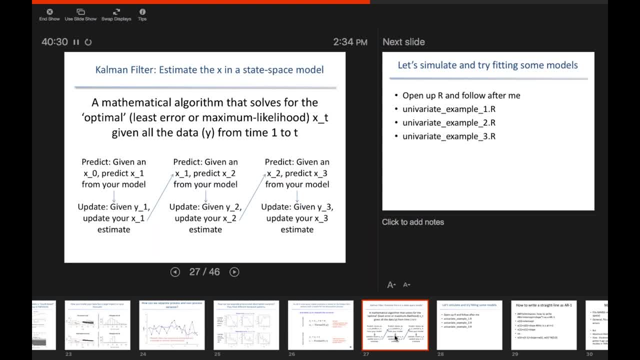 algorithm mentioned, when you definitely learn, you're working with this class of model. but also, if you were to read the help files for the ARIMA, you would see that they've mentioned the Kalman filter. And they mentioned the Kalman filter because they rewrite a. you know a. you know a. 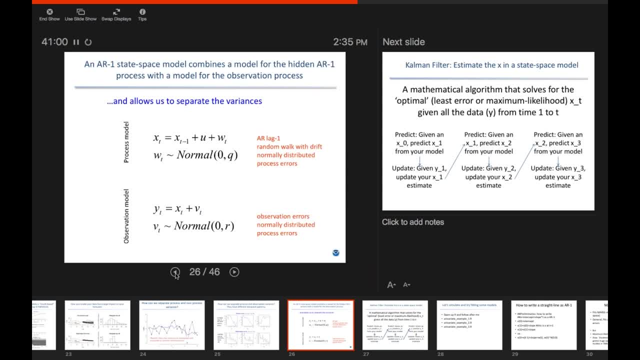 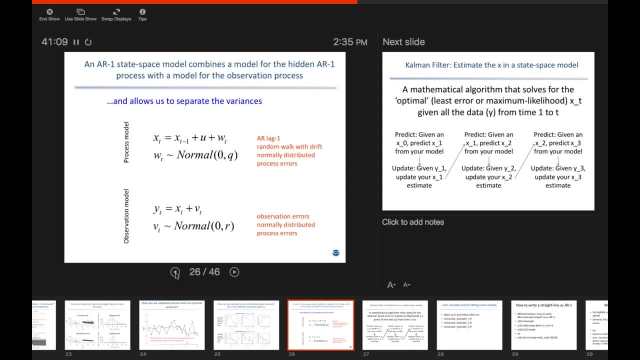 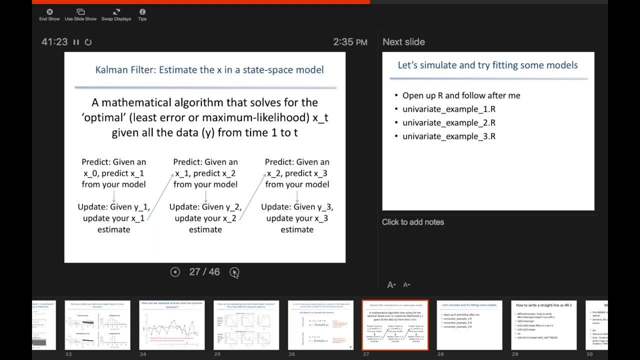 It's a matrix form. They write it as a state-based model of hidden state and observation And then they can use the Kalman filter algorithm, which is very fast. So the algorithm works basically like this: You predict the update, predict the update algorithm and you start at the beginning. 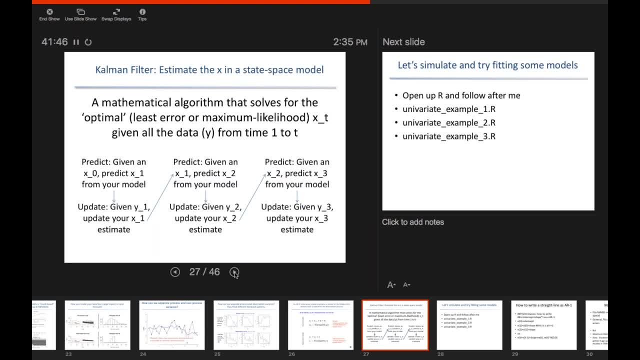 of your time series and then you're going to predict the next time point and then you look at the actual data that you've got and you update your estimate. So this is your prediction, given your data up to time t minus one, and then this is your 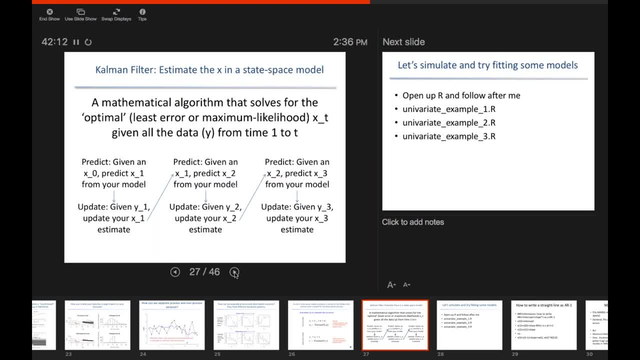 estimate of your state. You're estimating your state right. We have this hidden state, So we estimate what our hidden state is from our model and then we look at what the data were and then we're going to update. We update that estimate and then, using that estimate, we're going to make a new prediction. 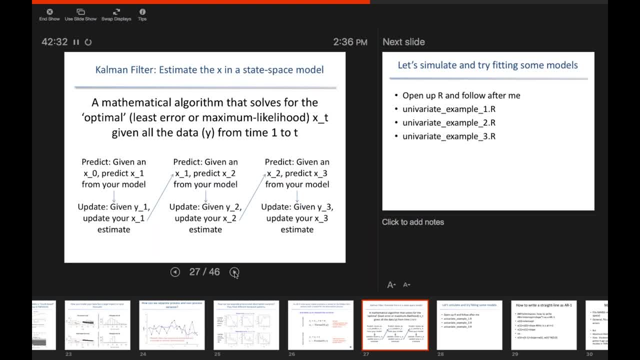 of the future and then we look at the data that we actually got and then we update that and then we keep stepping through our data And the nice thing about that is that if we want to make a prediction for time four all, 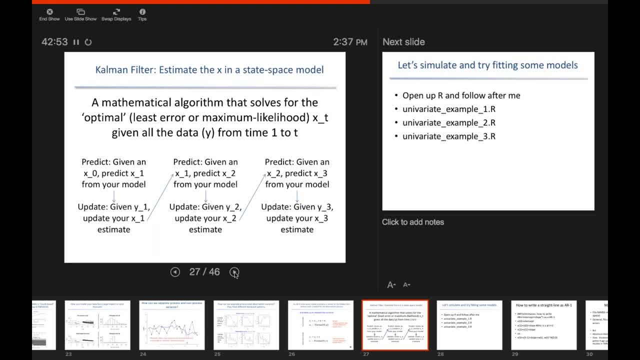 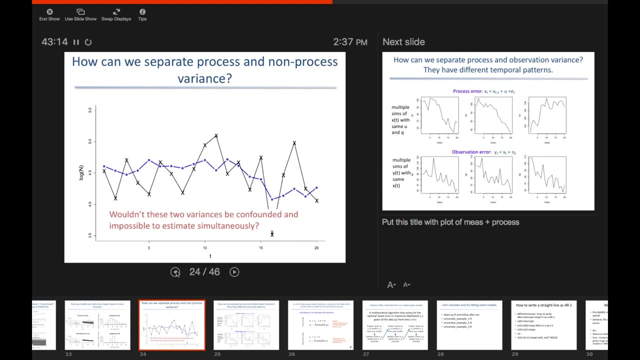 we need is the data from time three and we can make a new prediction. Okay, so whenever you hear the word Kalman filter being used, what you should be thinking in your head is hidden state. So I have a Okay. So I have a typo problem where I have some observations and there's this hidden underlying 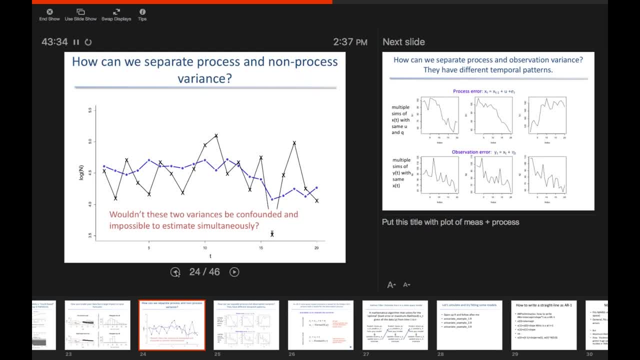 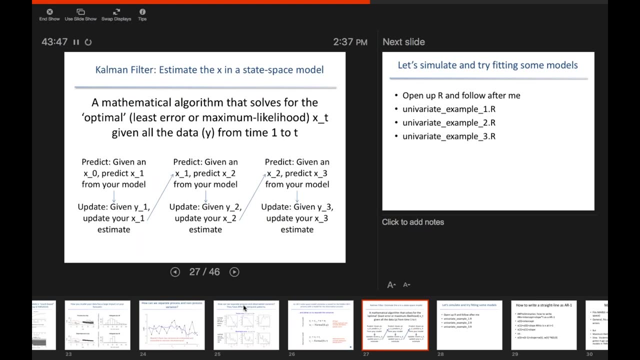 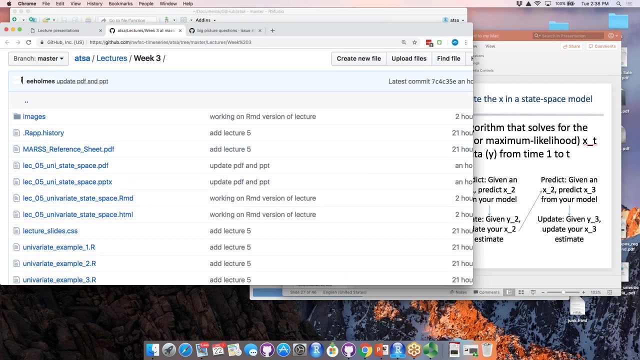 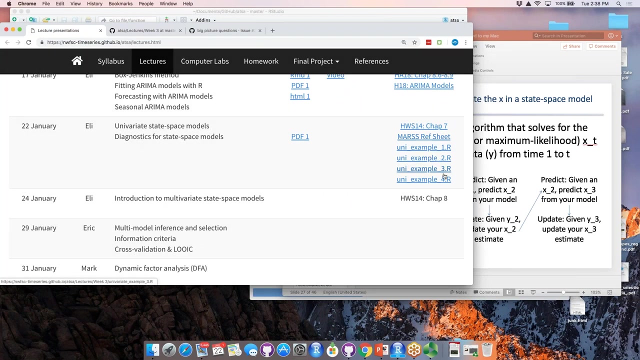 state and the Kalman filter is going to estimate that blue line. It's going to give me that blue line, Okay, so let's jump in and start trying this. So if you go onto the website, You see I have the univariate example one, two, three and four- and we're going to start. 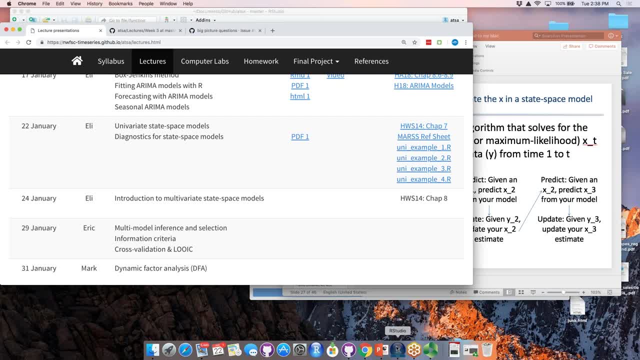 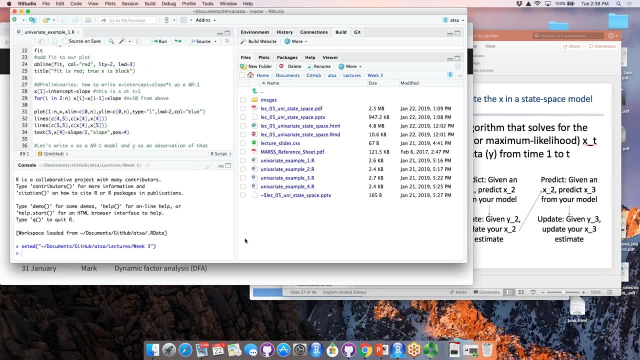 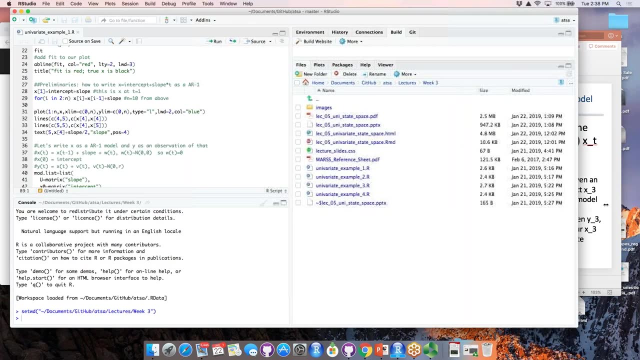 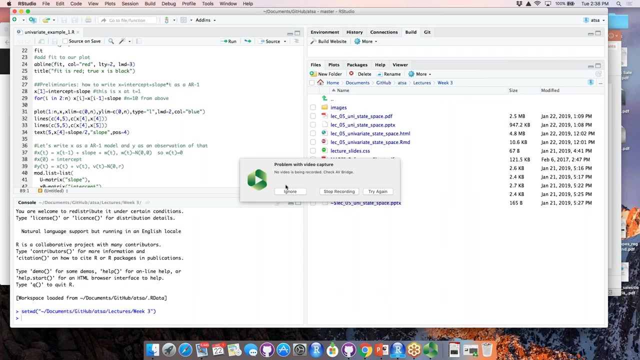 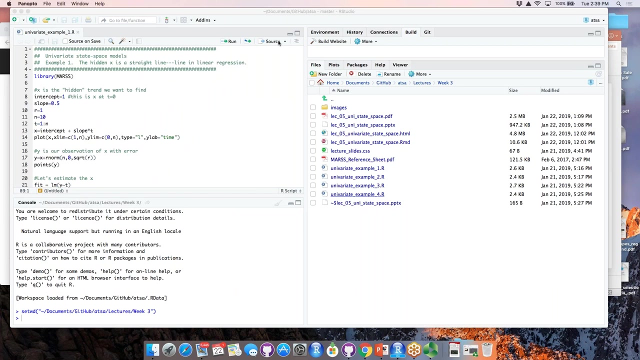 with univariate example one: Okay, Okay, let's make this a little bigger. So once you open that up, let's just Okay, Okay, Okay, Okay, All right, Thanks everybody. So let's just do it again. 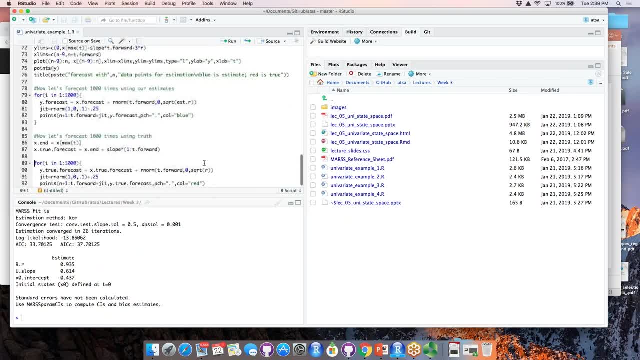 So what we're going to do is we're going to do a little table. So let's just do table a table first. Oh, that's good that we just do that. Okay, So that table is going to be that table. 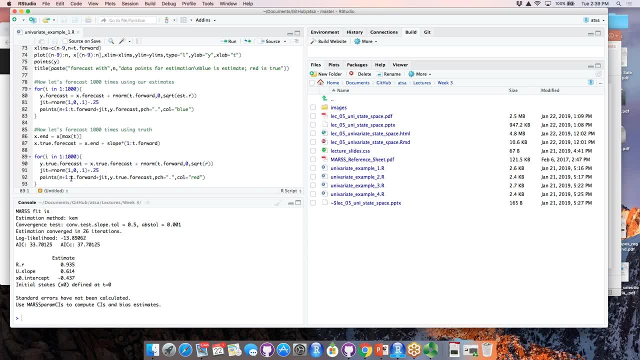 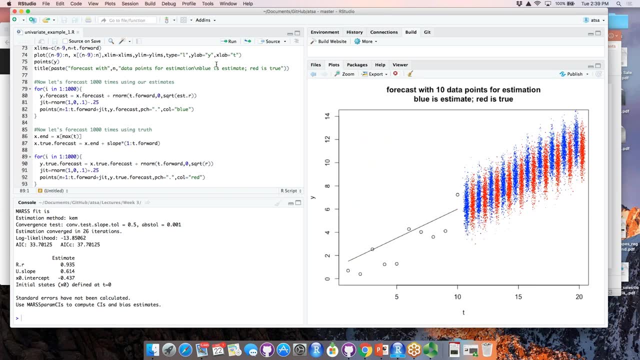 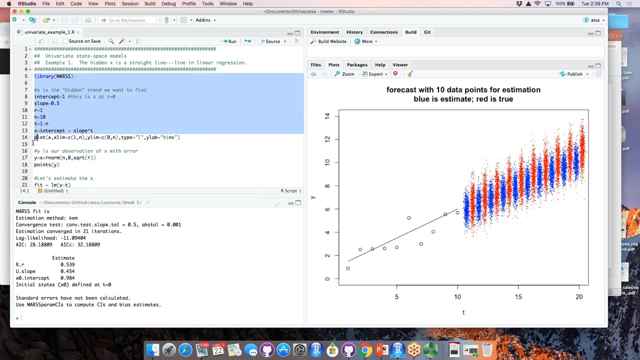 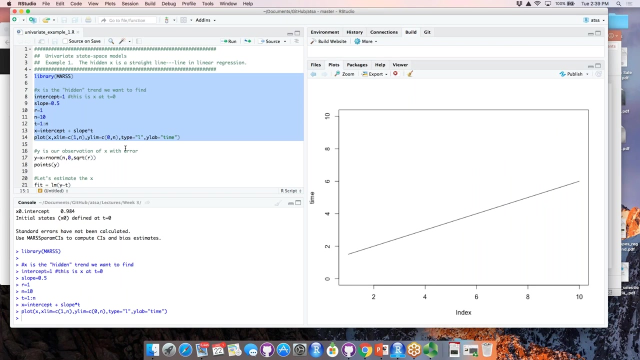 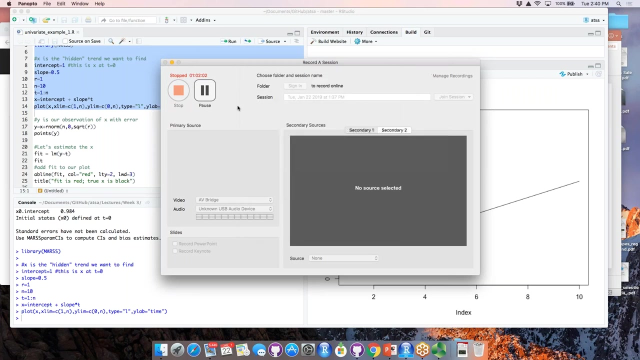 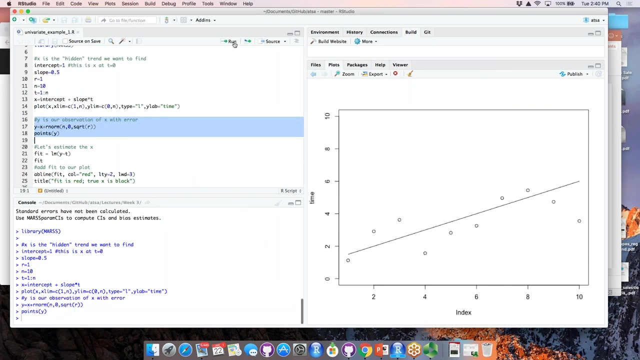 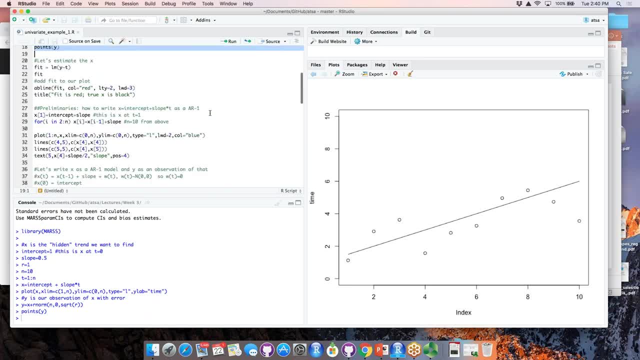 have some data around that line and then we're going to estimate that line using a linear regression. so it's the next block of code. okay, except really simple idea, right? okay, there's just a line and there's our data and the red is our estimate of that line. you see, it wasn't perfect, but we wouldn't expect it to be. 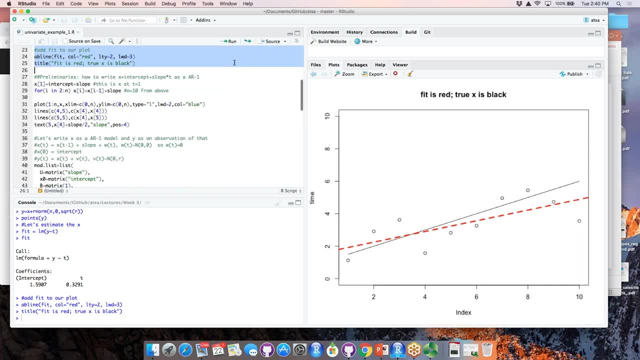 perfect. we've only got what? 10 data points there, and now we're going to fit this with a hidden, hidden state model. there's a couple on the floor, okay, so you want to fit this as a hidden state model. you want to fit it as something that looks like this: X, it was X, T minus 1 plus Q plus W, T and Y T. 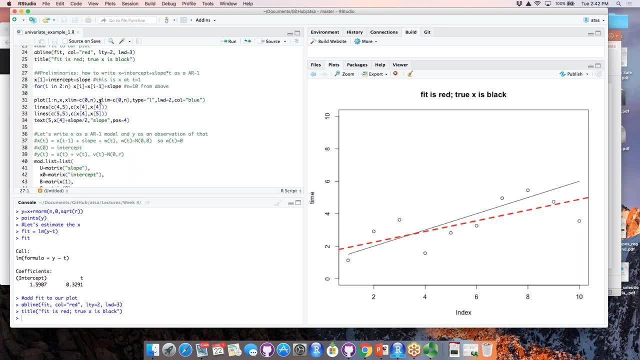 equals X T plus V T. so we need to figure out how to write that linear regression in this form and to do that we will have that X one equals the intercept plus smoke. those are in there and then we have X. have that xt equals xt minus 1 plus what do we have there? slope plus wt. 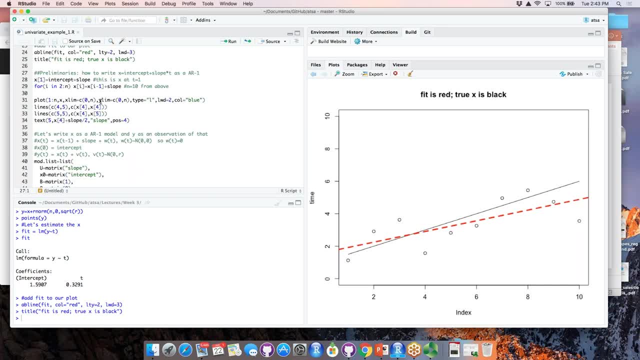 So that is here what a linear regression looks like. This is the important part: that you see that it's this plus the data point in the past, plus the slope, And the reason you need to recognize this is now you see how you're going to specify. 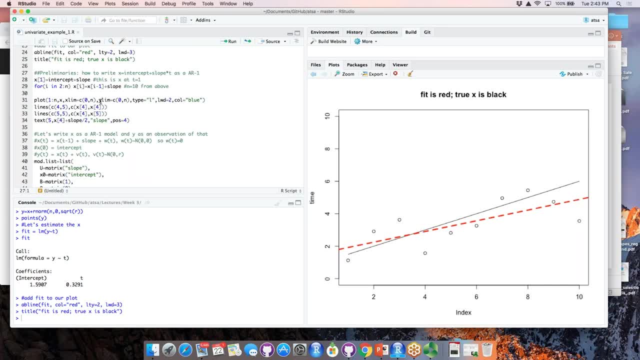 the model when you fit it. Okay. so now we are going to dive a little bit for five minutes into specifying the model for the MARS package, And the MARS package wants to know exactly what that equation there looks like, And Okay, 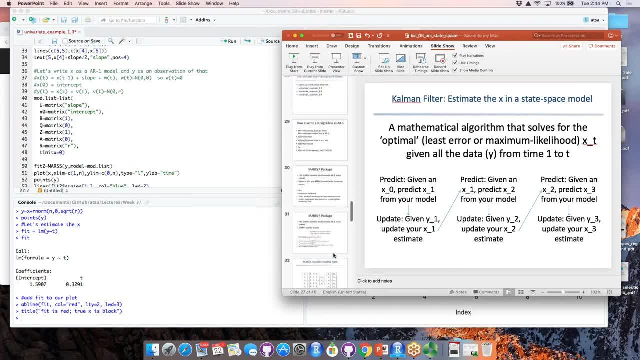 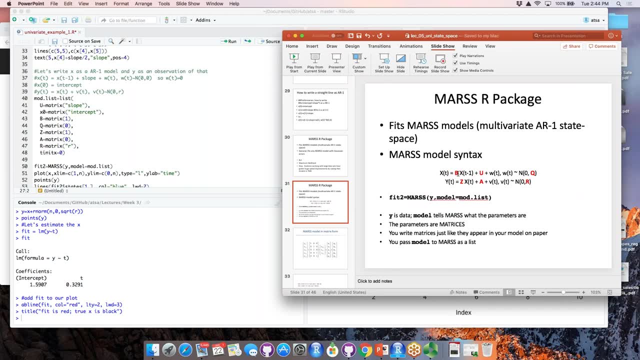 It wants to know what is that B matrix. So look at that equation over there. what is that B? It's just a 1.. And look over here we specify as a 1.. It wants to know what the U looks like. 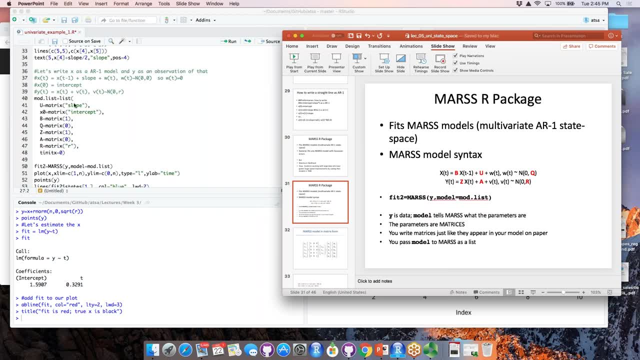 What is the U over there? Okay, that's slope. So we're just going to call it slope. It wants to know what the Q looks like. Well, that's something we need to estimate, So we're going to. well, actually, in this case, we're fitting a straight line. 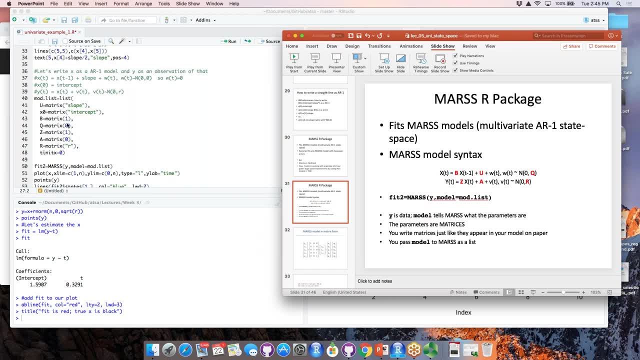 So that's just equal to 0.. So let's see, here We've got a 0, there, Now we've got to go to the Y. What does the Z look like? Well, it's just a 1.. So we specify that as a 1.. 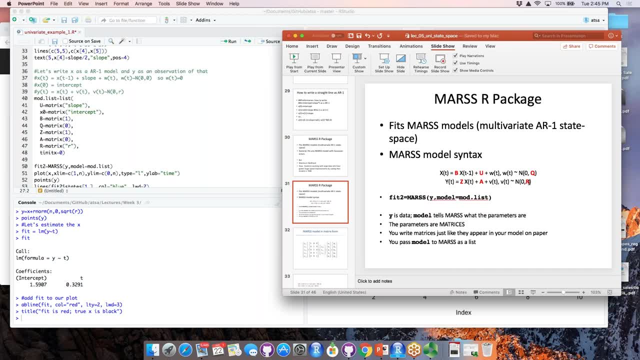 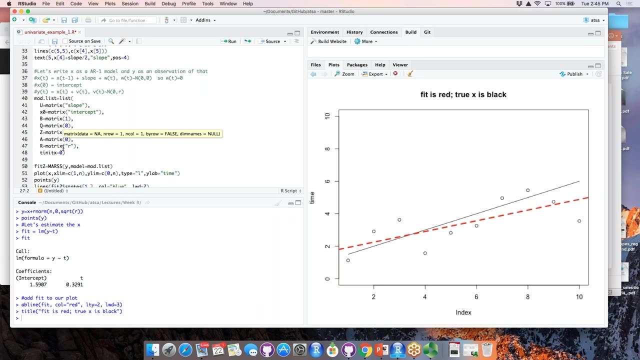 We don't have any A's there, So that's going to be 0.. And the observation error: that's what we're going to estimate right here. So this model list is that equation right over there. It's specifying what all the parameters look like. 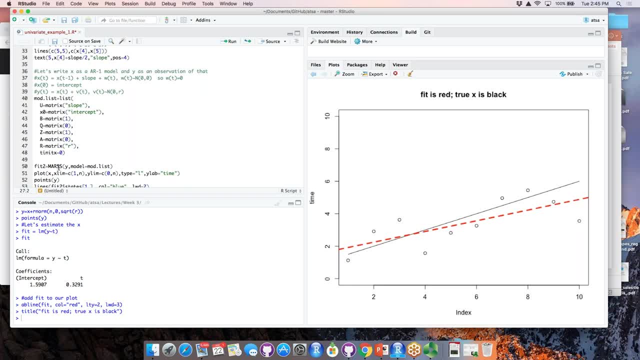 And now we can pass that in to this function, which is going to fit this model list, and it's going to fit it to that data Y. So now, to get this to run, you have to be able to install the Mars package. 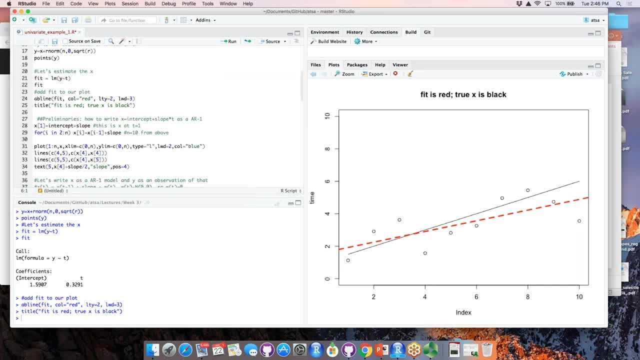 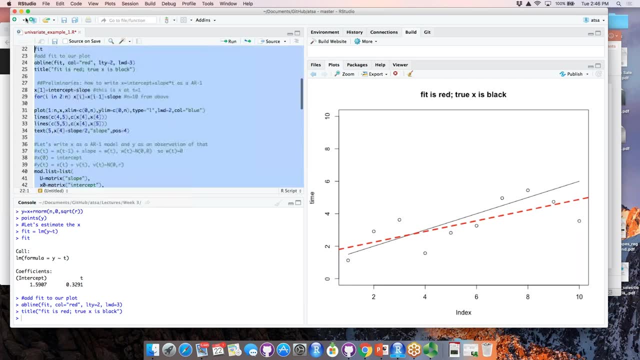 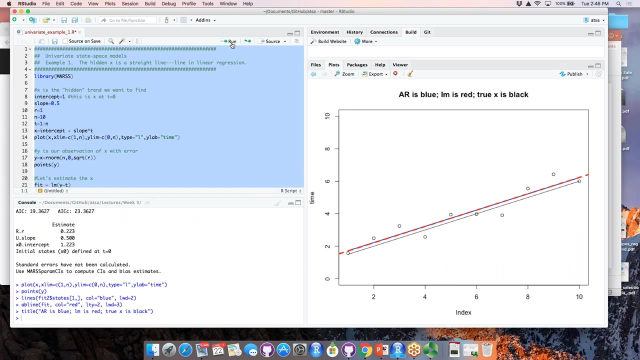 Let's go ahead and run this. So that's here, run all of that. see what that looks like. So it worked. So the blue line was what came out of the linear regression, out of the LM, And then the red line is what came out of rewriting that model as a state-based model. 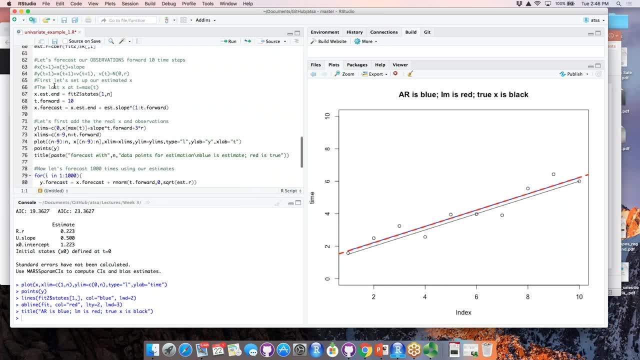 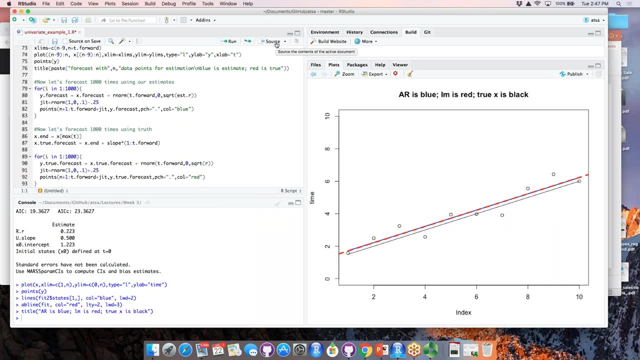 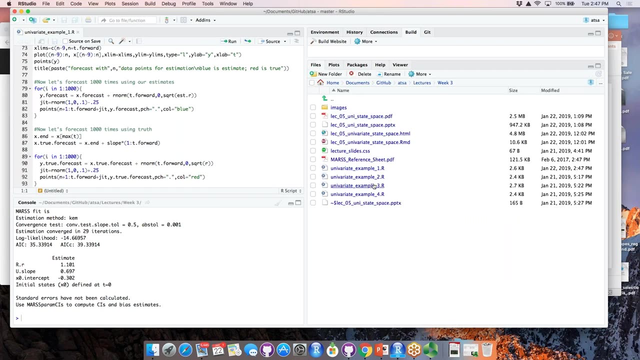 Let's go forecast. Okay, So that was the key bit I'm going to do. yeah, I just want to quickly do the next file, that's this one here, And this one is showing you the same example, same sort of example, but we're going to fit. 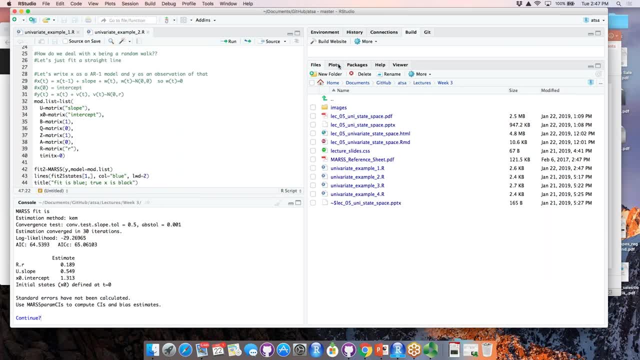 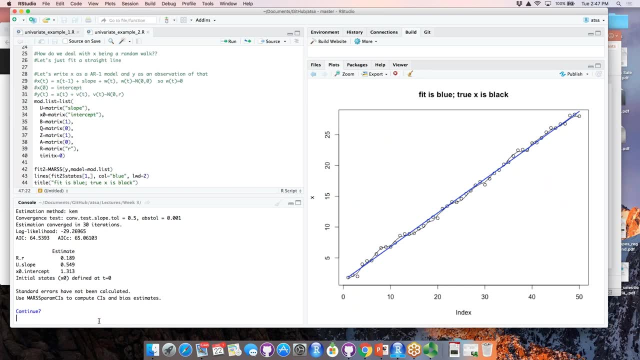 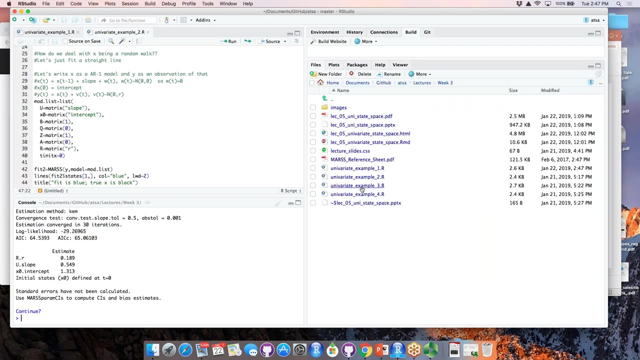 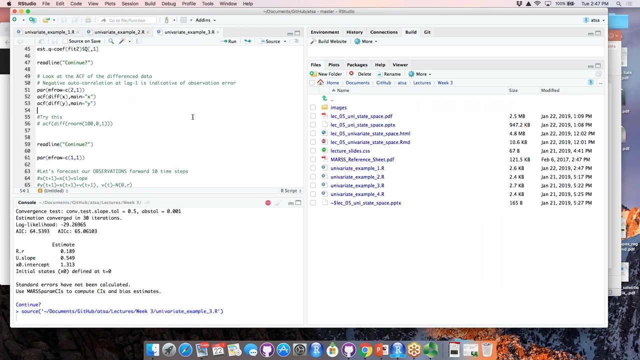 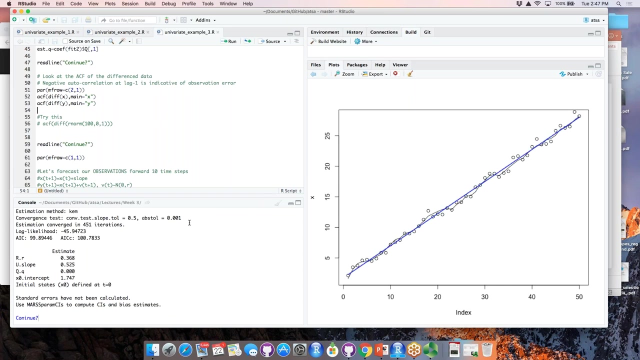 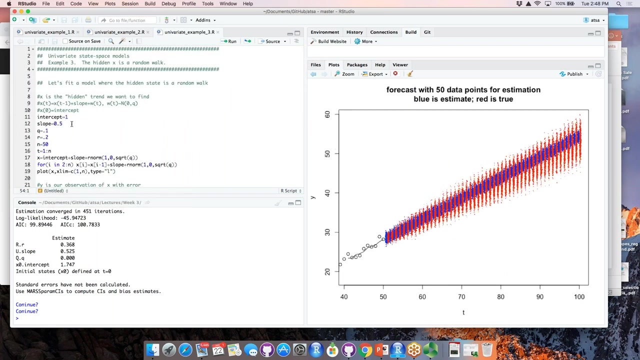 a random walk. All right, Let's open up three. Okay, So this shows you the example where come on. Okay, All right. So this is the example where you're estimating the hidden walk. Number three is showing you where you're estimating the hidden walk. 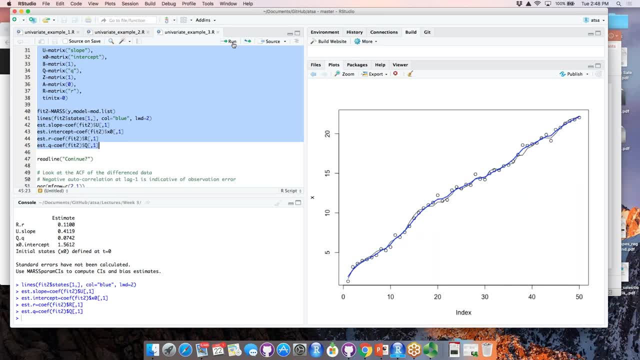 Okay, So what we have here is this black line is the hidden walk here And the blue line is what we have. So this is the hidden walk here And the blue line is what we estimate. And so, to fit this model, what we do is we need to specify this. 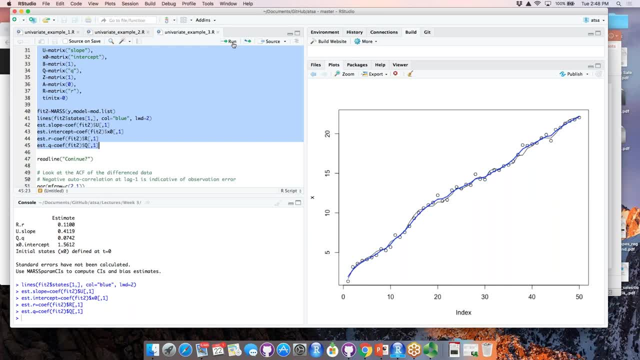 This is the random walk, but now we don't set this to zero. We don't set that variance to zero because we want to allow that to vary. Remember, for the linear regression we set that to zero, So it would be a straight line. 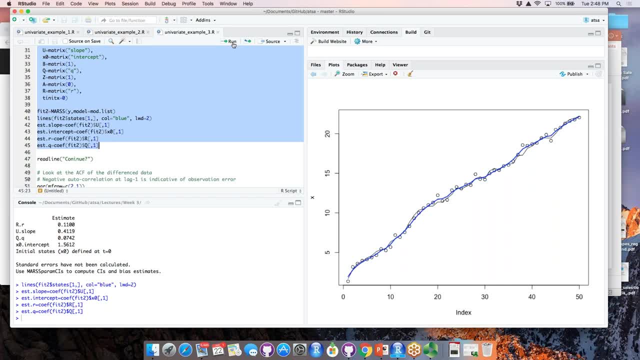 We allow that variance to be there And then we set that to zero to be there, and now it's a squiggly line. It's that random walk. We have that, and then we have our measurement, which is just the xt with the arrow. Let's look at what that 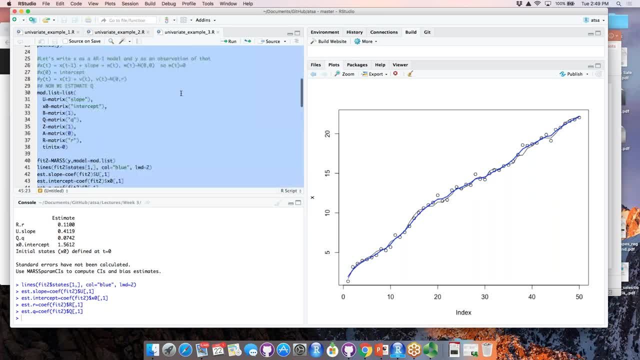 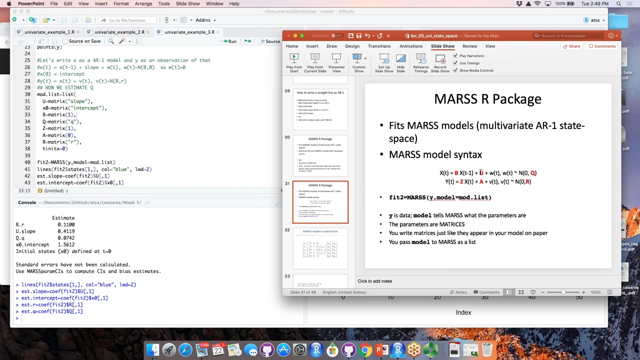 looks like in the R code. It's just translating one-to-one. We've got mu, sorry, the u. That's our slope. We've got an initial value. Ignore that. The key thing is here. we have this v, We have that v, That's 1.. We have that. 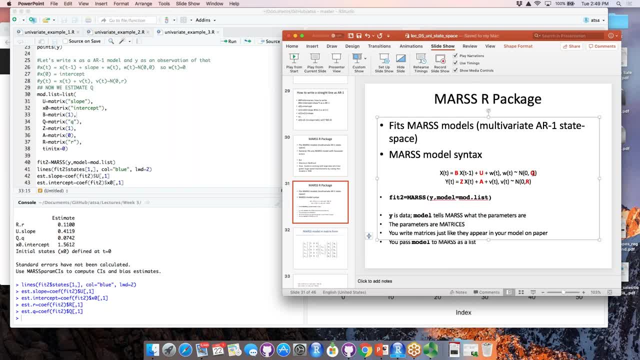 That's what we're estimating. We have the q. That's what we're estimating. It's right over here. We're estimating the q, The z is 1.. We set that to 0, and this we're estimating. This is exactly the process that you're going to be using for much more. 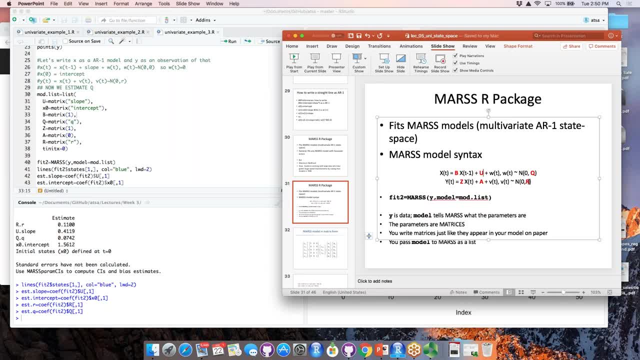 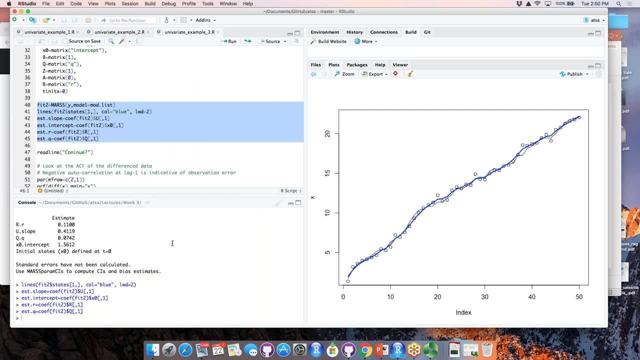 complicated models. You're just going to take this and you're going to start working through bit by bit what these look like. Then you can fit them here. And this is what it's estimating. It's estimating that the observation error is going to be 1.. And this is what it's estimating. It's estimating that the observation error. 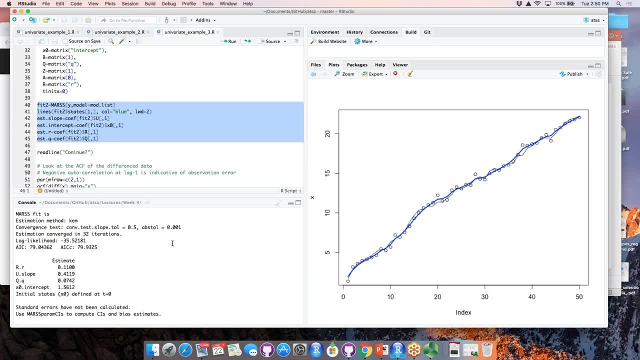 variance is 0.11,. it's estimating the slope is 0.4, and then it's estimating the process variance. All right, Okay, let's finish there. Go ahead and run through those four scripts. That's going to give you a lot of practice, just kind of running through these. 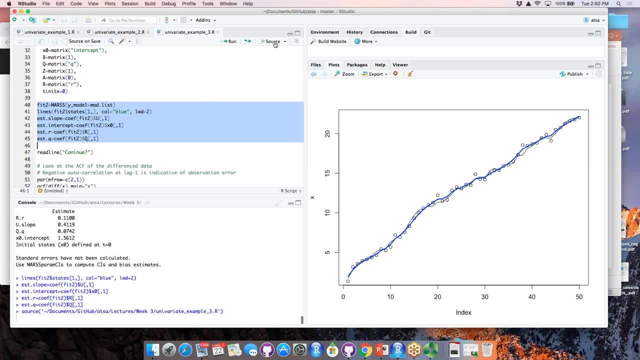 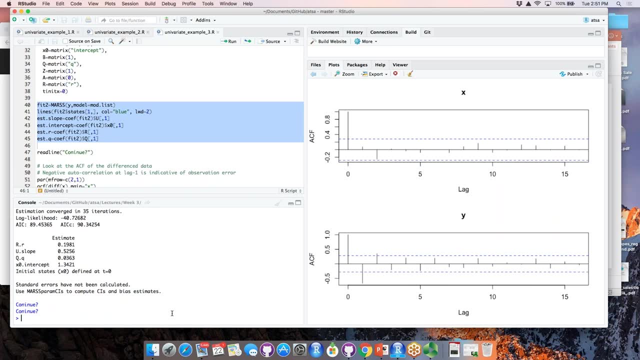 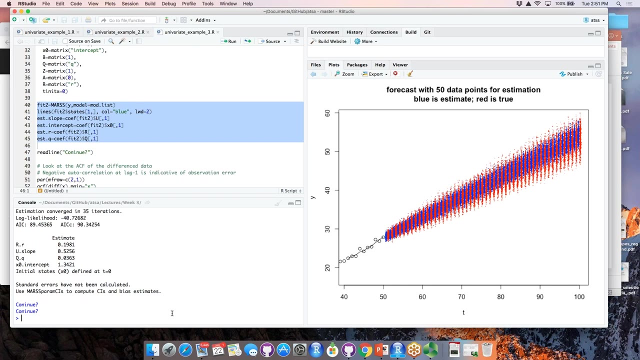 looking at the code. It's going to produce a variety of plots for you that you can sort of look at and think about, particularly these right here. This is showing you an estimated forecast using your estimated parameters, and red is what the true forecast should have been, And it's going to show you what those forecasts look like. 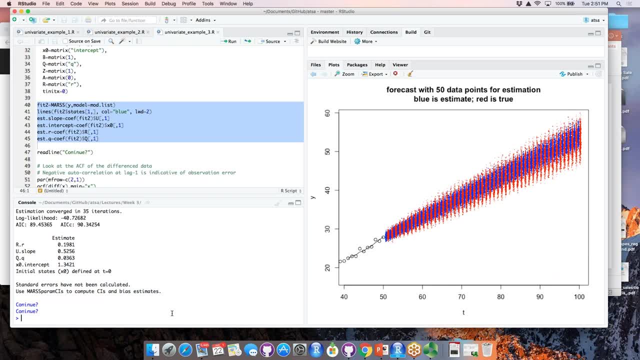 When you have a process error-only model and an observation error-only model and you'll see how very different they are.